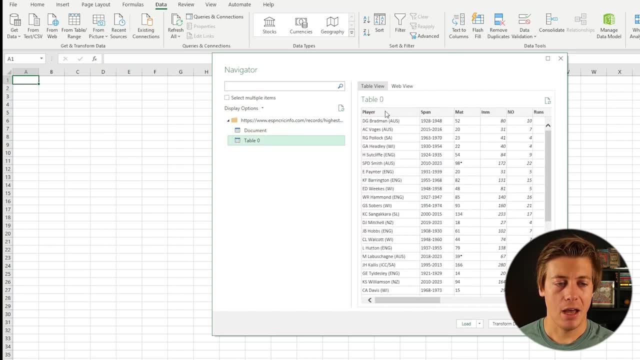 This is not what we want. but then if you go to table zero, you can see player span matches all the way over to over here, fours, sixes, hundred stocks, all that type of stuff. So this is what we want, And then all you're going to do is go down here. 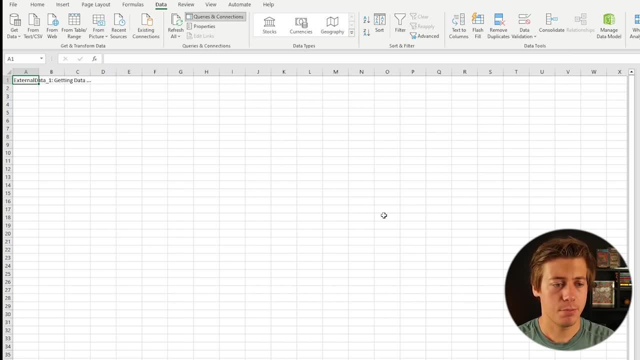 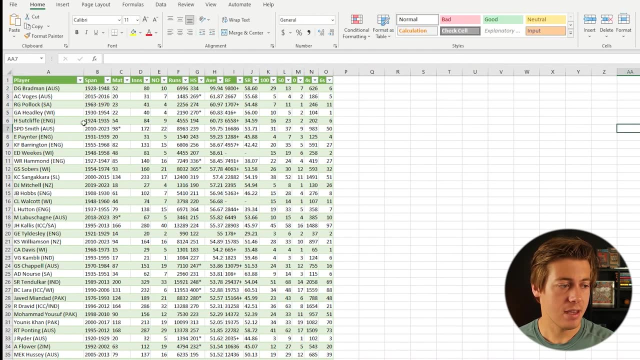 to load and then this is going to load into the spreadsheet. So now we have 63 rows loaded, which is really cool to see, And this is how it is specifically built out, And I already know there's going to be a few things that we're gonna have to work on. Um, so you can see, like over here. 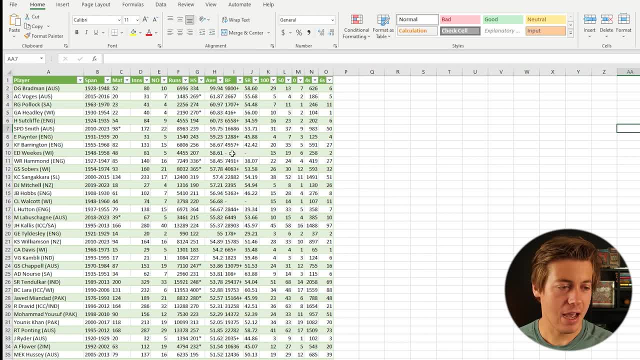 stars. and then over here: um, we have some dashes, we have some plus, but I'm going to update a few things in here, um, just to make this video a little bit better, All right. So instead of these dashes here, I'm just going to leave these as blank. Uh, that way they show up. 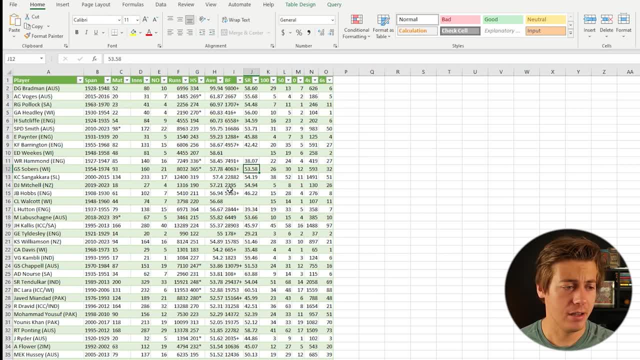 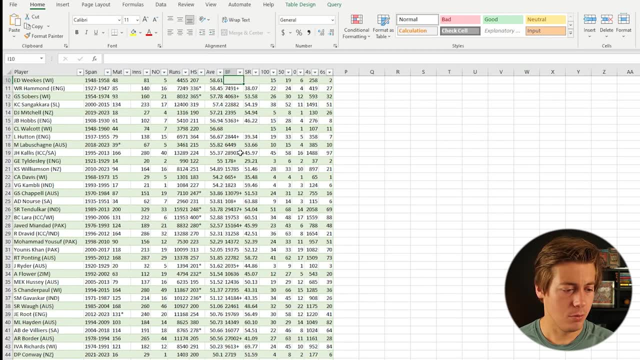 as null and we can uh transform this data. I'll show you a little bit later. It's kind of interesting, um, that these have no specific data in here, but I will figure that out. The other thing I want to do is: 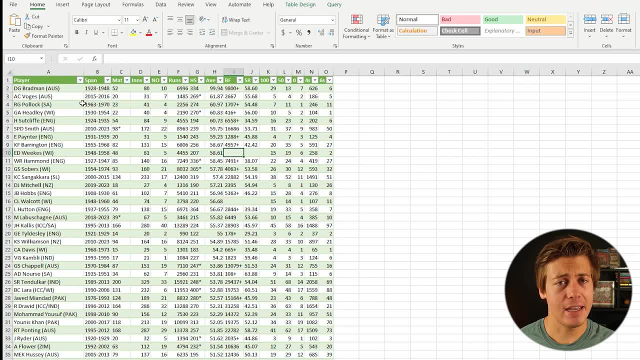 make a few duplicates. That way I can show you how to drop duplicate data. Uh, sometimes it does happen, when you're either extracting data or you know you get a spreadsheet or other form of data. Sometimes records are duplicated and you're going to have to be able to solve that. So 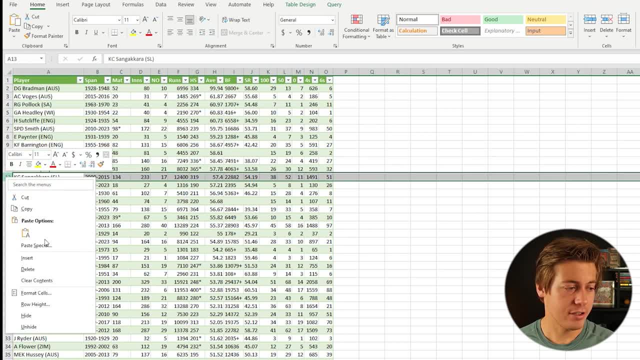 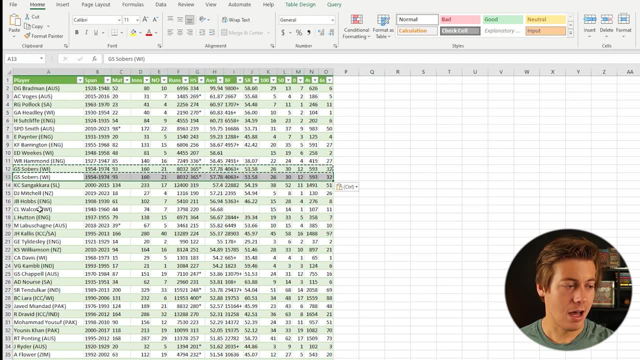 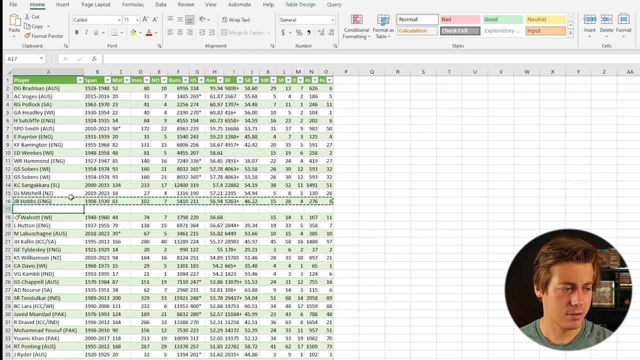 I'm just going to copy a few different names over here. So we have the legendary Gary Sobers. I'm going to duplicate all his stuff over here. We can put that over here. Hobbs as well, very legendary. So we're going to grab Hobbs, but over here probably top five cricket player of all time. 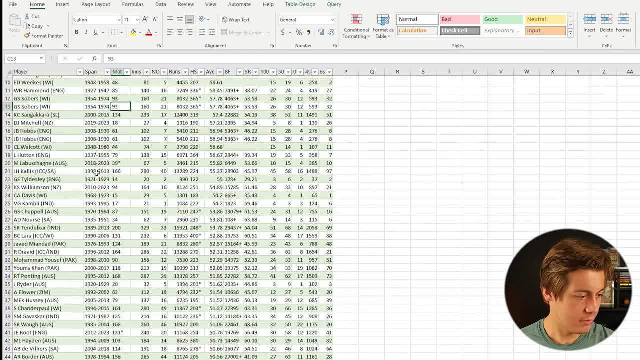 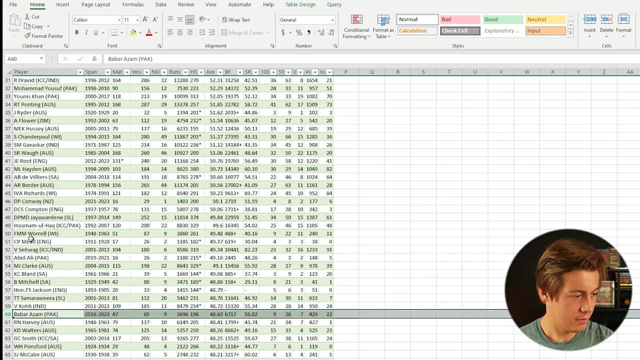 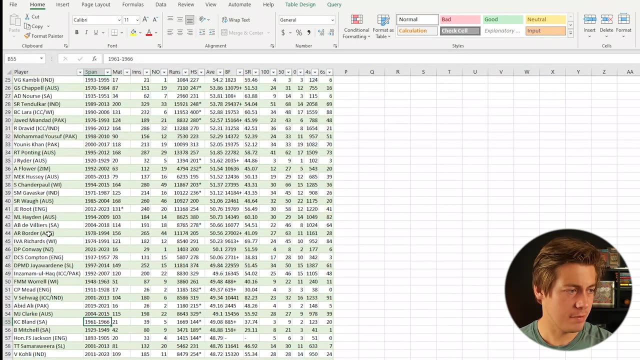 And then let's grab one more. So let's just go over here and see who else is in this list. Um, grabbing this over here and we have three that should be duplicated And I think that'll be fine. uh, for this example, 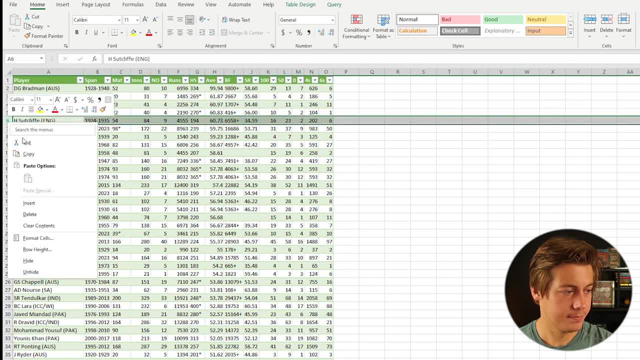 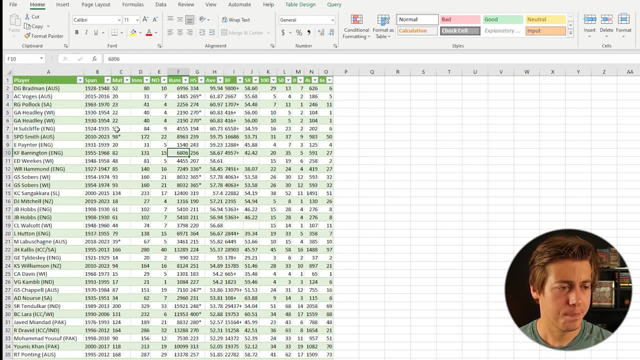 And, uh, let's do that. Oh, we'll do one more headly as well. So I'm still looking for one of his cards. One has two of his. I do not. So, uh, we have four examples of players that have duplicated data. Uh, so now you want to save this. 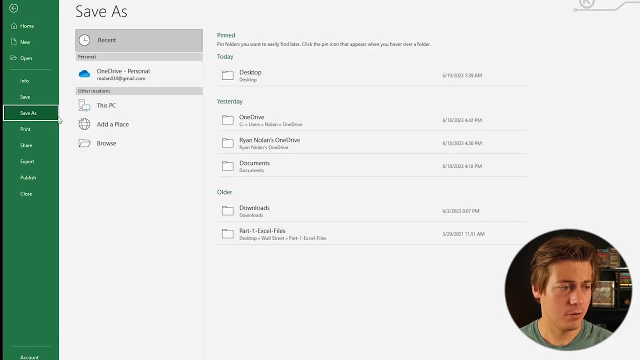 as a CSV. So I'm just going to save as and then I'm going to put over here and you're going to want to make sure to save this as a CSV. So you see cricket test match data. We see CSV dot there. 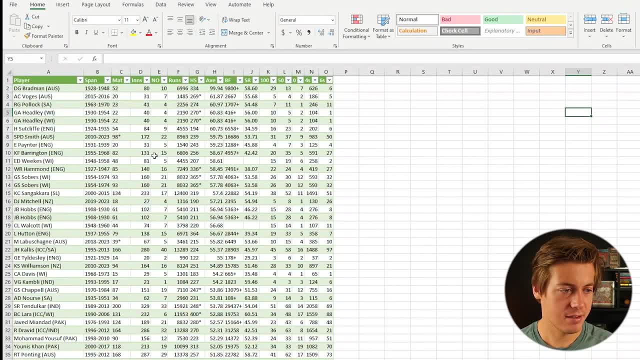 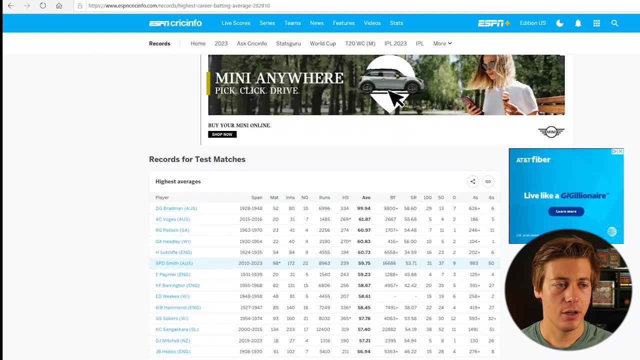 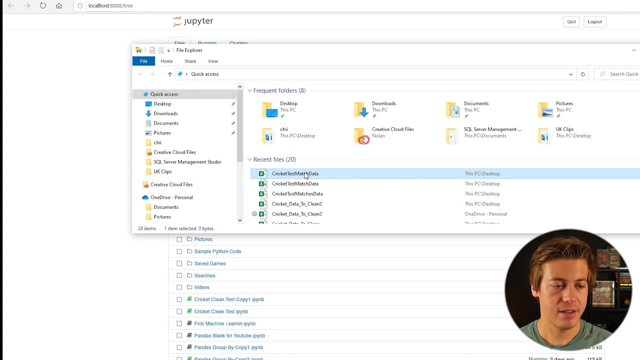 and I'm just going to label this dot CSV like that, And we should be good on that side of that Things. So next we're going to want to drag this into our Jupiter. So I have this over here, the mean Jupiter screen, And then I have this over here, uh, just on my desktop, So I'm going 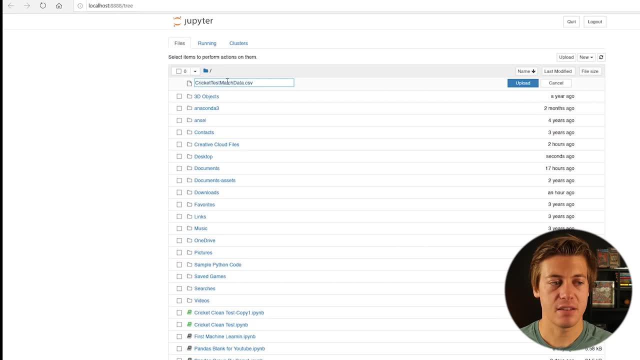 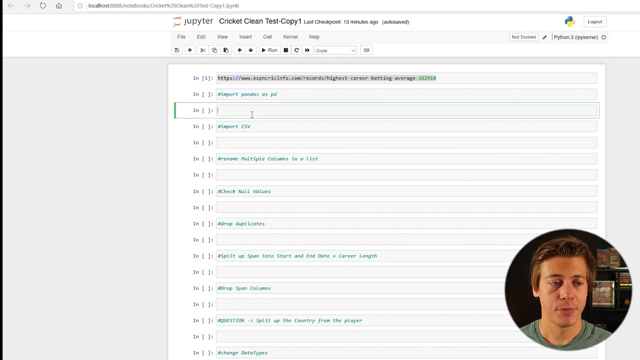 to drag this over here and then you can see it says cricket test match data dot CSV, and then click upload And now that has been uploaded, So we can actually import this in here, And the first thing that you're going to want to do is import pandas. So I'm just gonna say: import pandas as. 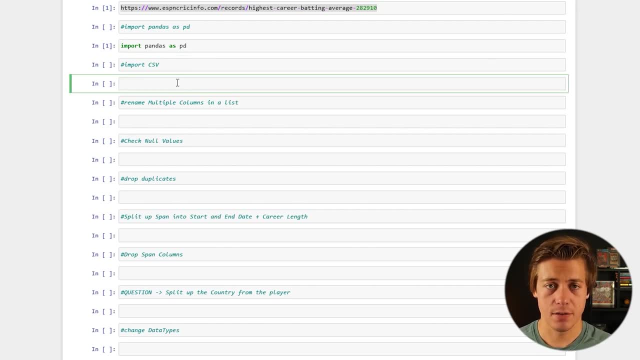 pd Always do that. And now we can import this CSV, So I'm going to just call this DF. So we're going to say DF equals pd, dot read CSV. And then we got to grab the name of it. So if I just go to last, 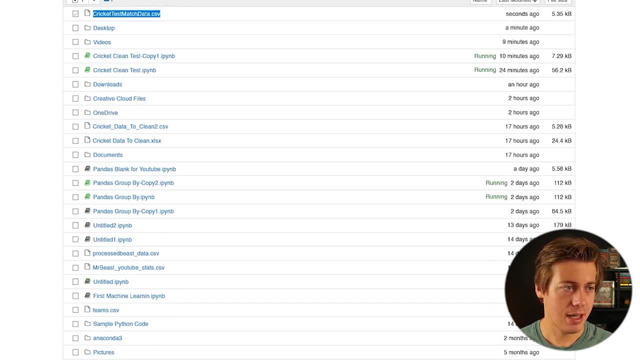 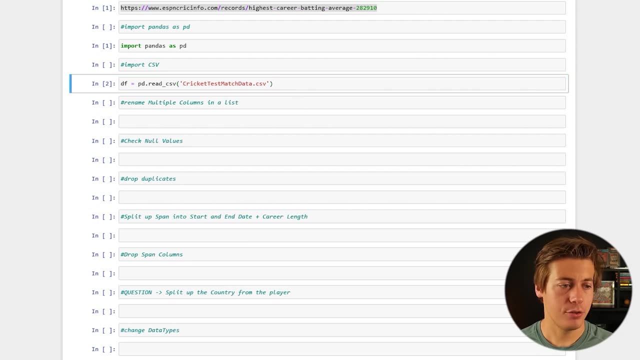 modified. you can see it's like this. So I'm just going to copy that and then throw this in here And to make sure that this works properly, I'm just going to do a new line and I'm just going to put DF in here. 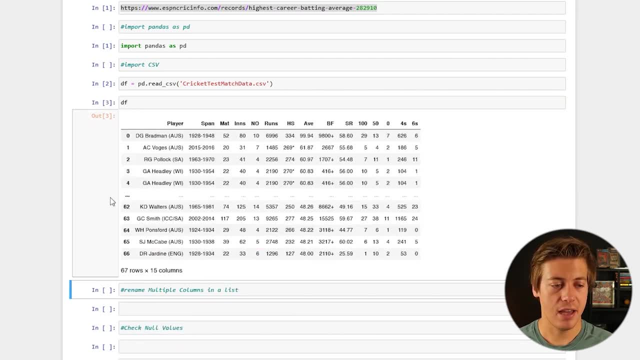 And let's do that, And you can see that this has been entered. Now, if you don't know what I'm doing to run these, instead of going over here each time, I'm just clicking shift enter, So that allows you to run the specific. So now you can see all of this data is on here, which is: 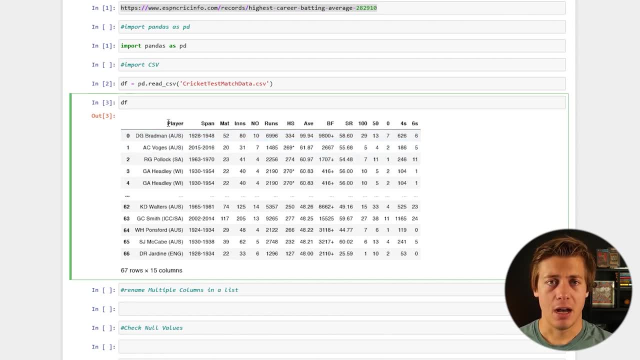 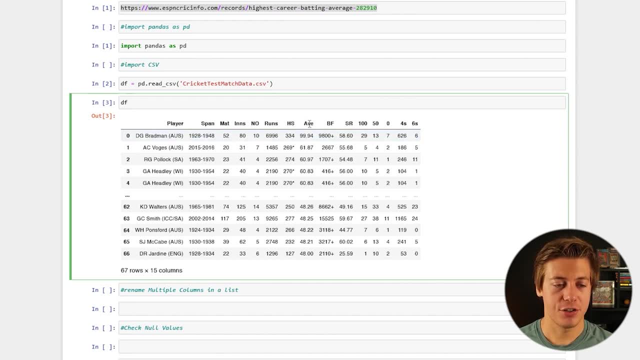 Like this just says: no, this is HS, I'm average, Makes sense on there. Uh, BFSR- like what does this mean? Uh, so let's re name multiple of these. So what we're going to want to do first is type. 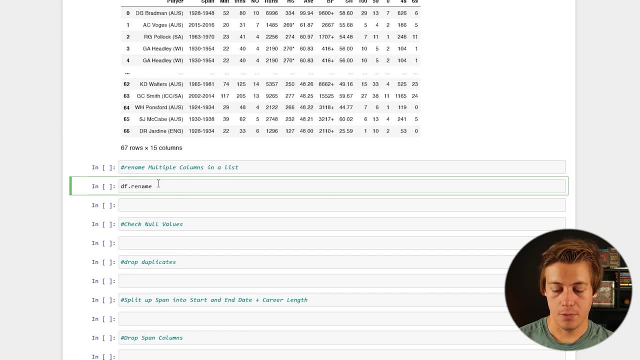 in here: DF dot rename- And then what you're going to do is open this up in here and you're going to put columns equal, and then you're going to just build out a list, right, And what we're going to have on this side of things is the first column. 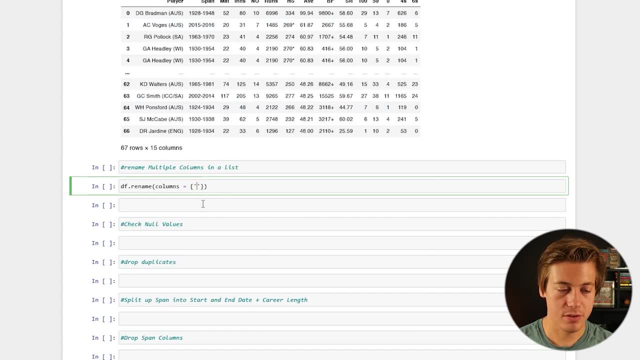 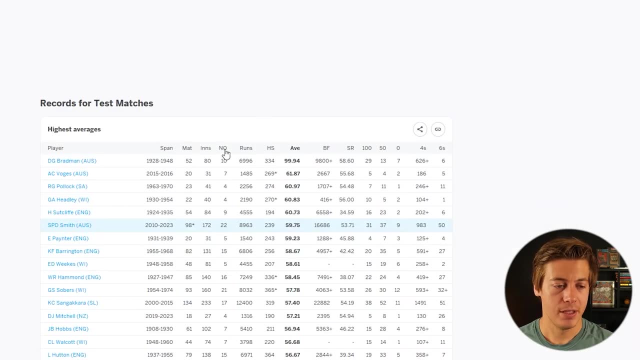 Right. So like no, I'm going to say like this: put single quotes. No, I'm going to put a colon and then we're going to put the actual name. So if we go back over here, right, it says no means. 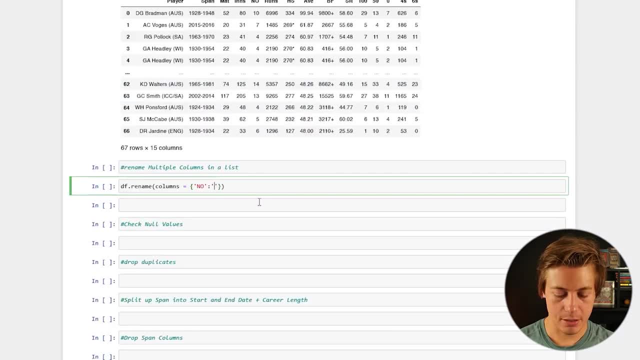 not out. So let's put that, And what I recommend is: you just do like this, Don't keep a space in there, because it can get pretty annoying. Um, but pretty easy. Now, if I run this on here, we're going to just see how this would change it. but this isn't assigned yet to the original data. 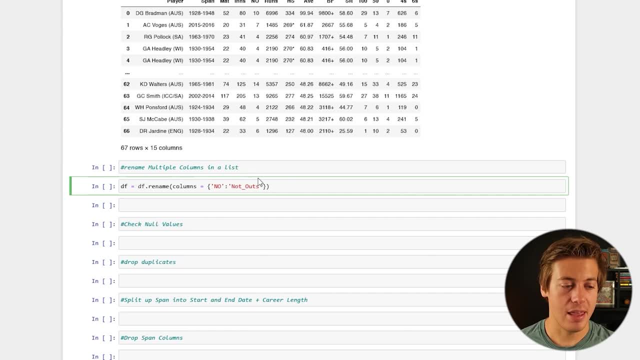 frame. Uh, to do that we have to put DF equals, and then we're renaming all of those. but I would like to rename multiple, So we already have that. The next one I want to rename is HS, So I'm going. 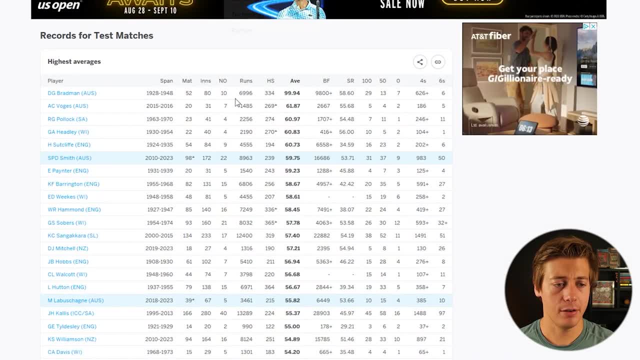 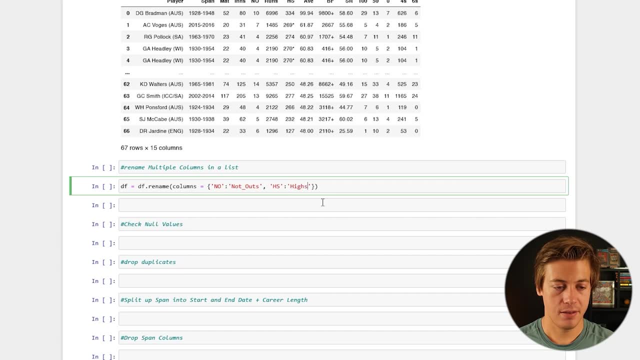 to put HS over here. And if we go back over here, HS is highest innings score, So we'll just put highest score. Okay, Let's go to the next one. Next one: So we have BF, which I think is balls faced. So we go back over here, balls faced. So. 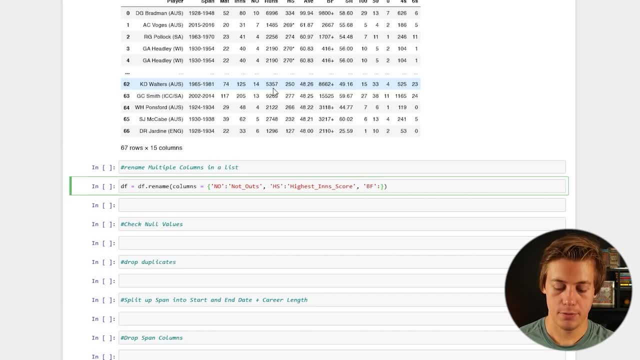 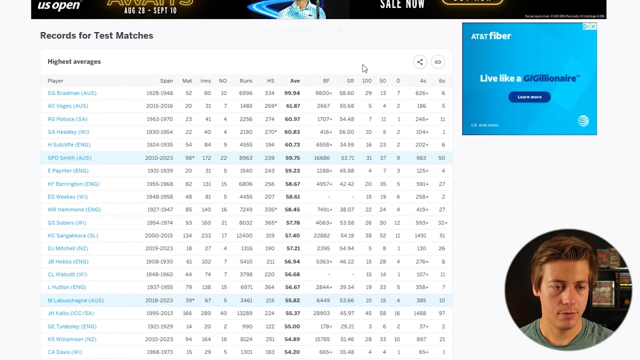 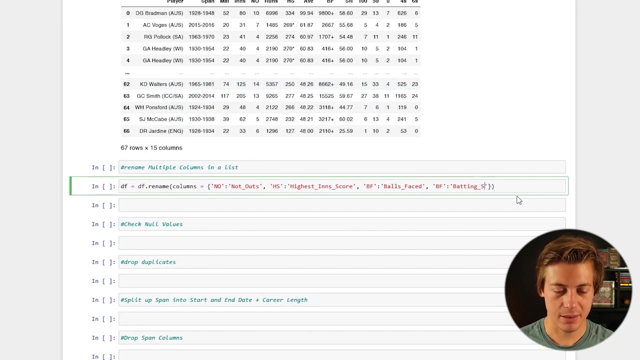 BF over here, balls faced, Okay. And then the next one, SR. and then we have SR over here is batting and strike rate. So we put that over here and then it's BF batting. And I was. and that's not BF, it's SR. That's why I was like what the heck strike rates? So SR, like that. 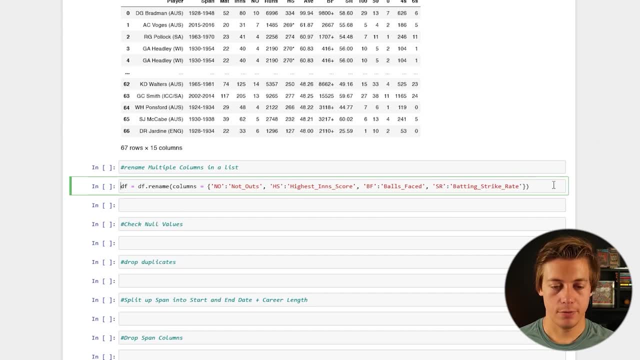 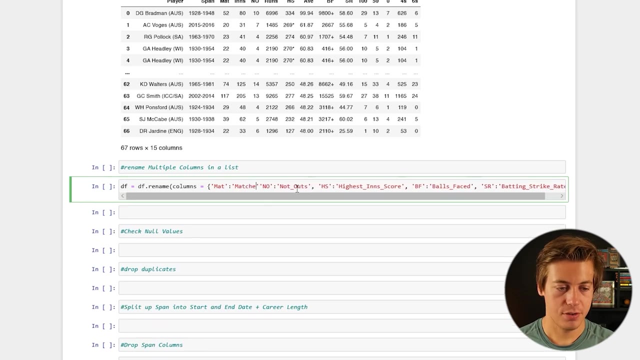 So now, if we run this over here, just make sure match MAT for matches, I think that's. eh, we'll put that over here too, Right? So we'll say MAT like that And we'll just put matches, Which is doesn't hurt to get a little bit more practice. So we have all of this now, right? And 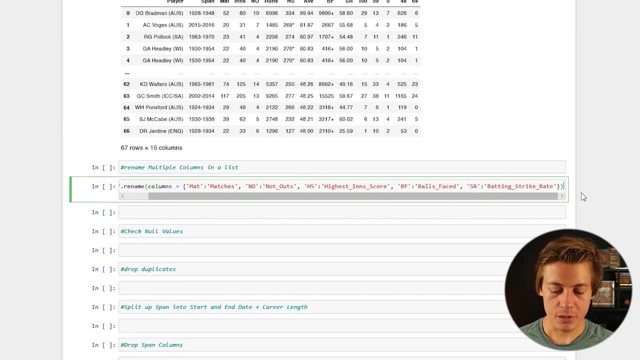 it's a little bit long, but that's all right. So I'm going to just do a shift enter And since we assigned it back to our original data frame, DF, we should now see this over here with the new information. So if I just put DF over here or DFhead, a lot of people just put DFhead right. 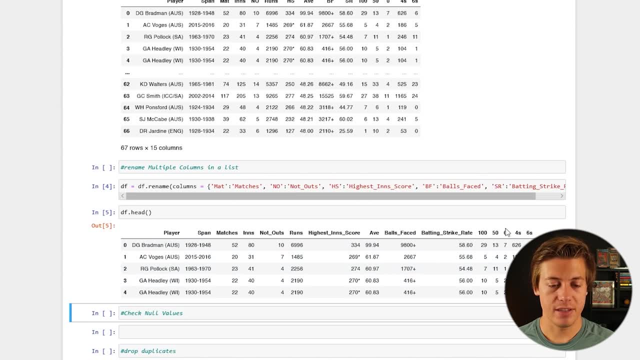 This will show the top five And you can see. all this has been renamed and obviously it's going to be a lot longer now than what it was over here, Um, but that's good. That means our renaming has worked. Now we're going to. 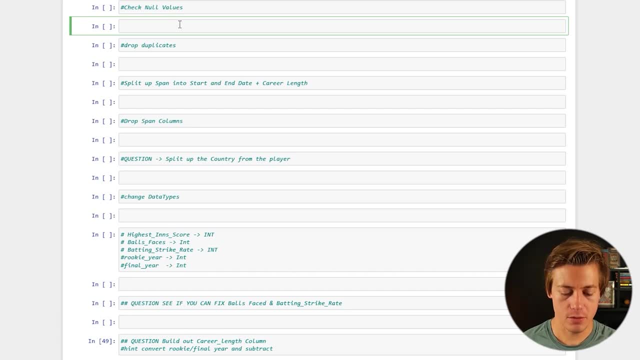 check for null values. Uh, so the way, easiest way to do that is you can just put DF and then you can put is null, like this, and then we're going to put dot any, and this is going to show us each of the 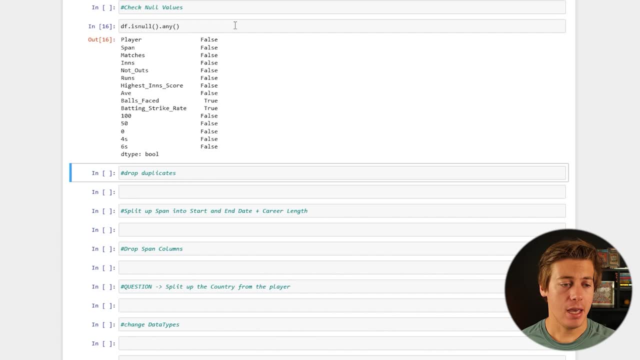 series is if there's going to be any null value specifically in it. And you can see we have two that are true. right, We have balls face. I'm going to open up a few more of these cells and let's kind of investigate that. So the easiest. 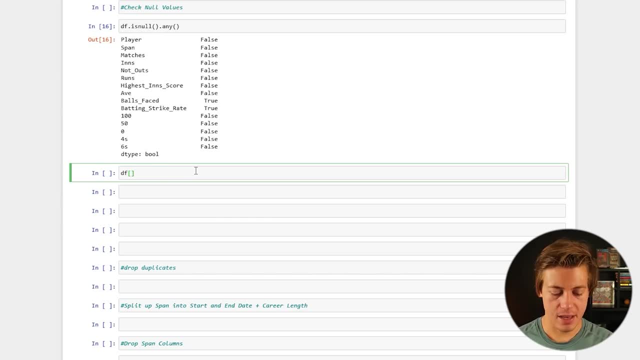 way that we can do is we can do DF like this, and then we're going to sit inside, We're going to put another DF and we're going to just put this first one balls face. And we can put that like this: And I'm just going to say that this dot is an A which will, which is very similar to null right. 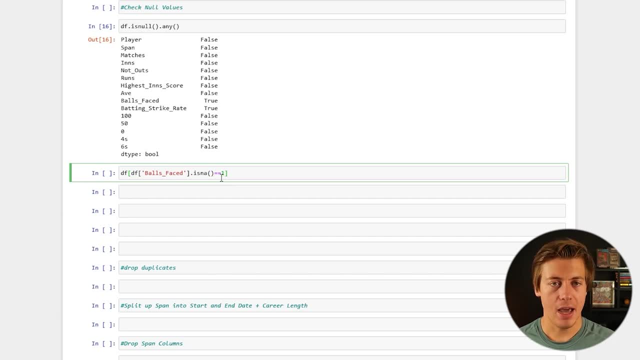 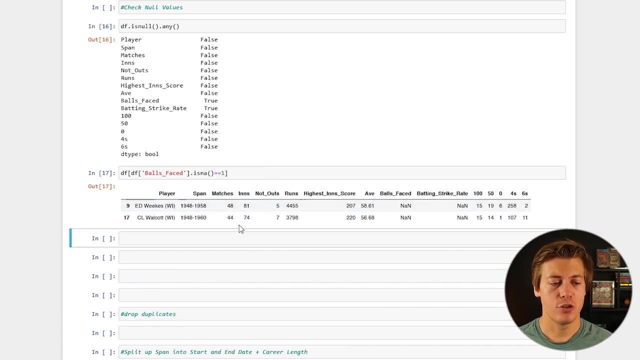 It's going to show true or false, So I'm just going to say: equals one, And this is going to give me the entire row output. Uh, when balls faced is null, Uh, so you can see that we have two of these right. We have Ed weeks batter's face and batting strike and and Walcott just. 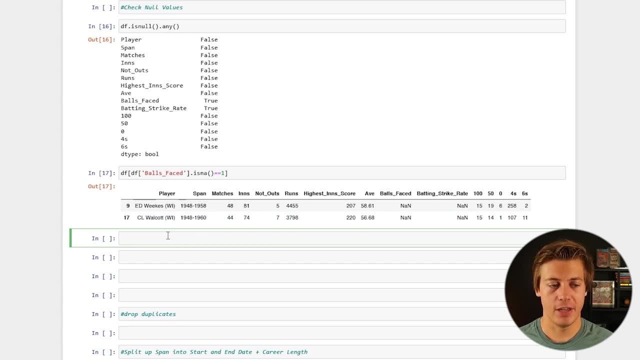 like our spreadsheet, So let's fix these. So the first one we're going to do is like this: So I'm just going to say DF balls, face equals, and we're going to say the same over here. right, Uh, but 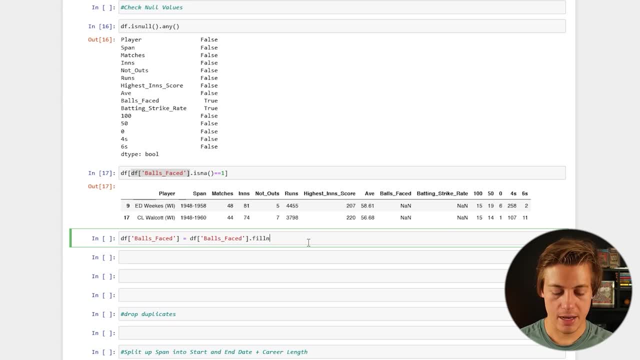 this time we're going to say um, dot, fill and a, and we're going to just going to put a zero. Is that probably the correct way? Like 50, 50.. I don't know why this data didn't populate, but we'll put. 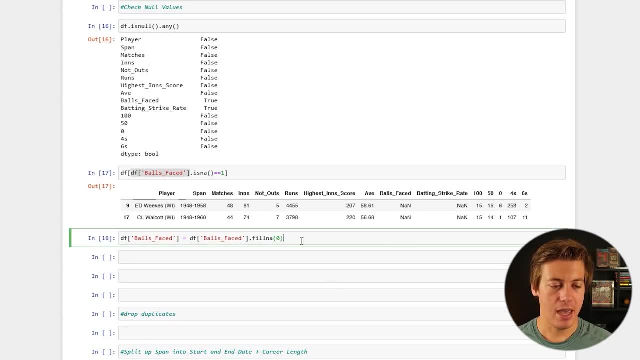 that in here, Right? And now that's been entered and let's do the same thing for batting strike rate. So just going to put that in here and then let's run that, And now let's run our data frame on the side of things, And 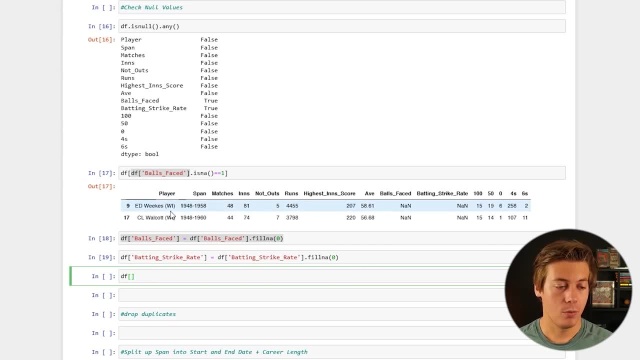 Speaker 1. Speaker 2. Speaker 1: For this data frame. I'm going to grab the player weeks over here. So what I want to do is put another F in here. We're going to say player and we're going to say that is equal to, and then we're going to just grab this And we're hoping. 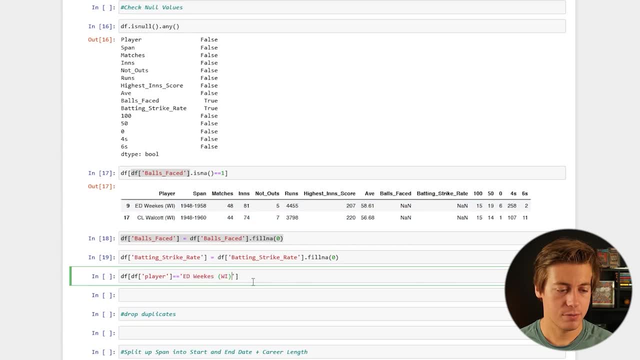 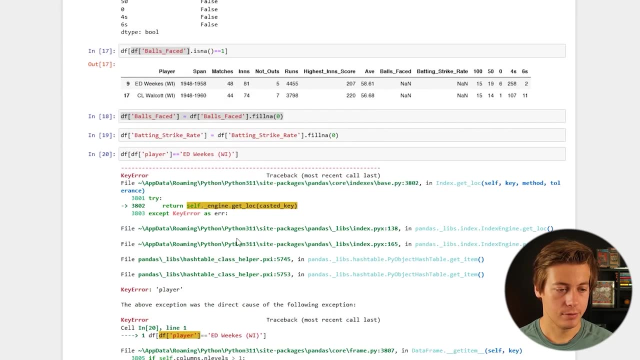 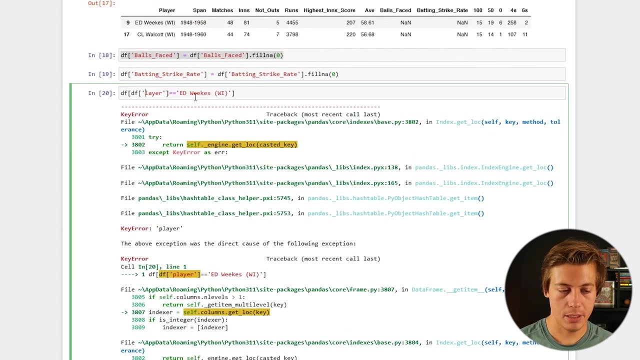 that these two values over here are now going to be zeros, So we just put that over here, and this should give us our full row, And we have an error on here. Let's see what it is. Speaker 2: This player is wrong and that's because it's supposed to be a capital P, So let's put that. 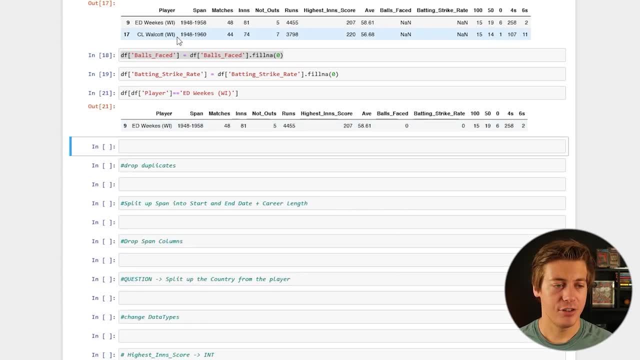 over here And now you can see it's zero for both of those. And just to play devil's etiquette, let's put wall cut on here. So grab that and put this on here and you can see that is also zero. So we successfully replaced these NAs with zero, which is good, because now 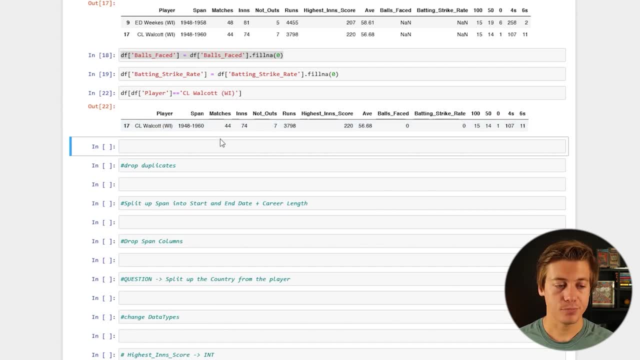 we can run some calculations on these columns if we really wanted to. But now I'm going to show you guys how you can drop duplicates in here. So I'm just going to remove that one cell and we're going to open up a few for the duplicate side of things. So what we can do first is put dfduplicated. 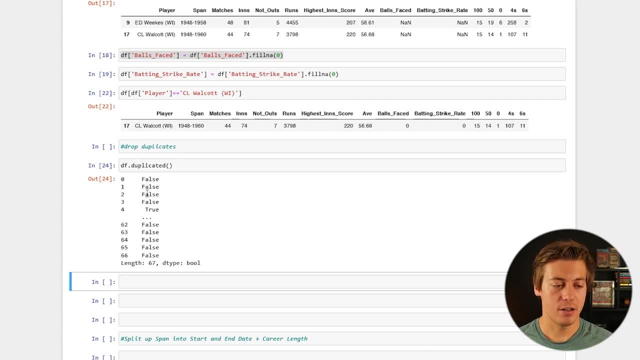 And if you run that you can see that most of these are going to be false. but we do have trues and it's starting off with four And that makes sense because we updated that spreadsheet to have a few duplicates, So kind of like before. 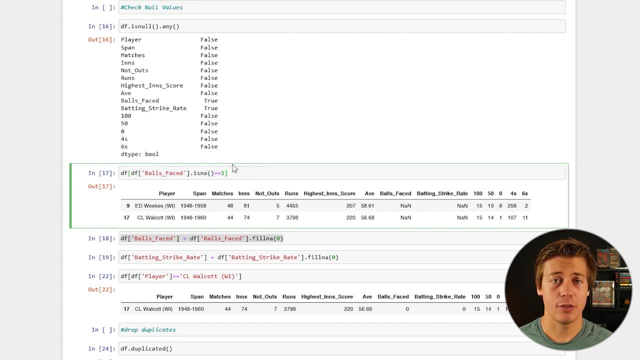 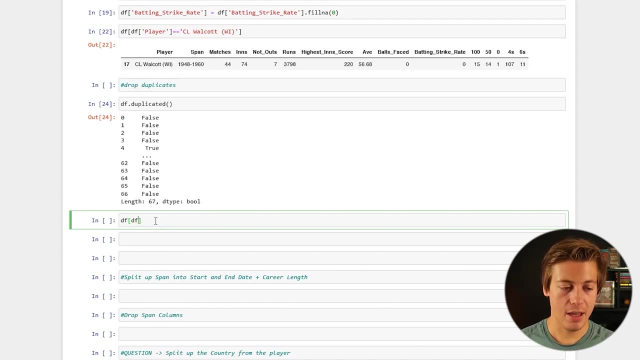 we try to figure out what's NA. We're going to do the same thing with duplicated. So all you have to do on this is I'm going to say df, Open this up, df. And I'm going to put player in here- Make sure it's a capital P so you don't get an error. And then I say dot, duplicated. 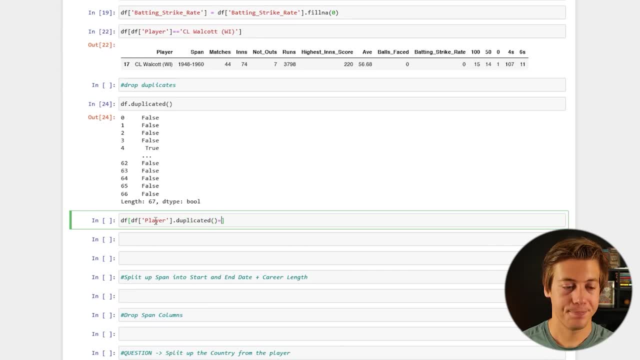 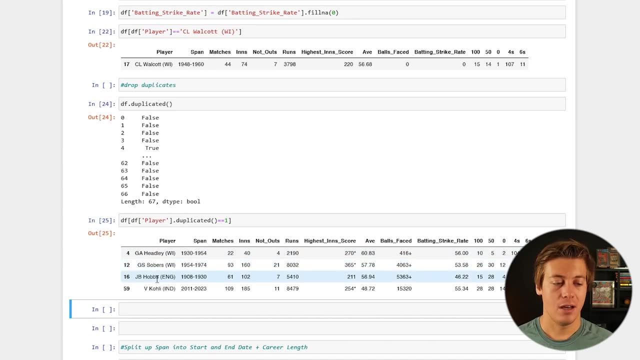 like this And we're going to say that's equal to one right, Like that. And then you can see we have four duplicates: Headley, Sobers, Hobbs and Coley- And if you wanted to show all eight results, all we're going to do on this case is we're going to 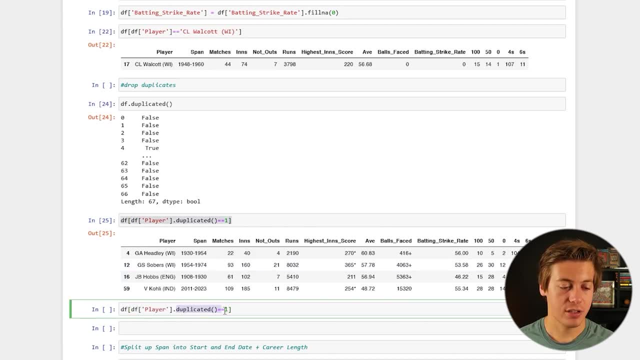 copy this over here Instead of dot duplicated. we're just going to put that is in, And then what we're going to do is throw all these different players in here. So watch all I have to do, All right, All right. 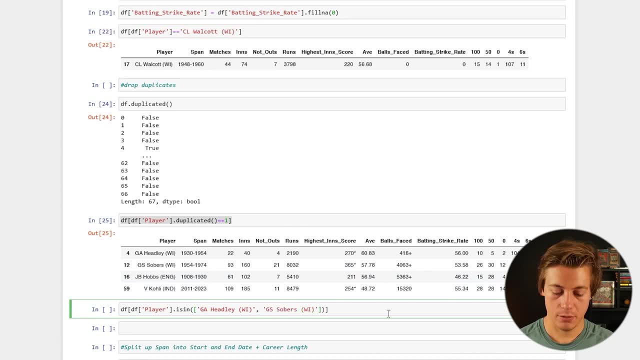 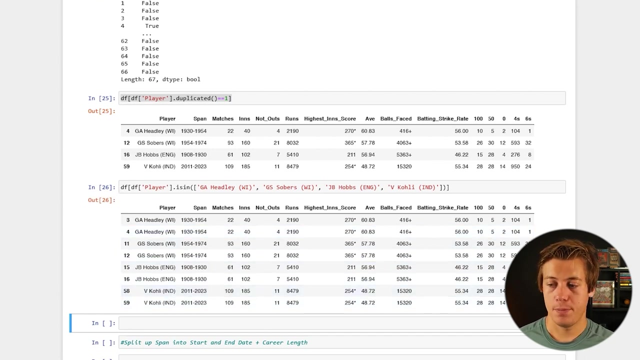 Just keep going like this And like this. So now when I run this, you can see there's going to be eight results, So Headley, Sobers, Hobbs and Coley. So not good right, Or this has all been duplicated. 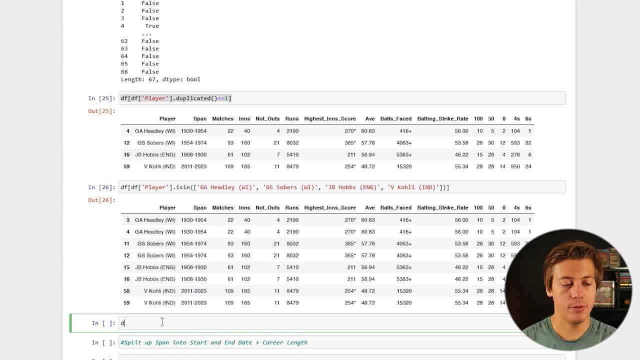 But we can try this. We can drop these now. So all I have to do is df dot, drop underscore duplicates, Duplicates like this, And this is going to drop the different rows. So now you only have one of each of these. 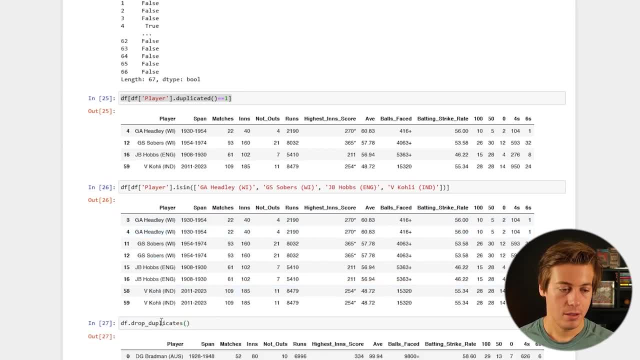 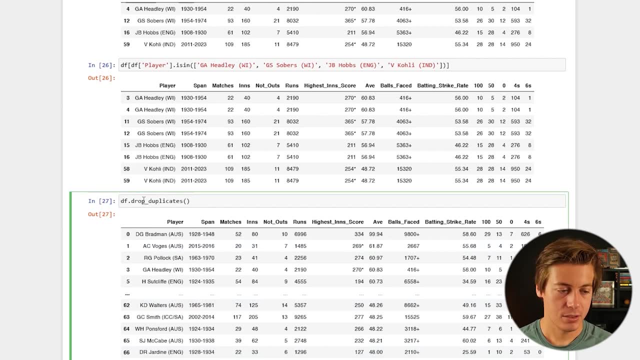 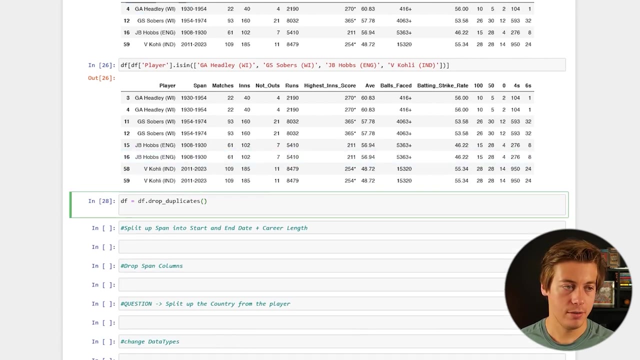 So we run that. You can see our data frame now is to 63. But we have to assign this back to our original data frame. So just put df equals df, dot, drop duplicates And then what we're going to do is run the same one as above. 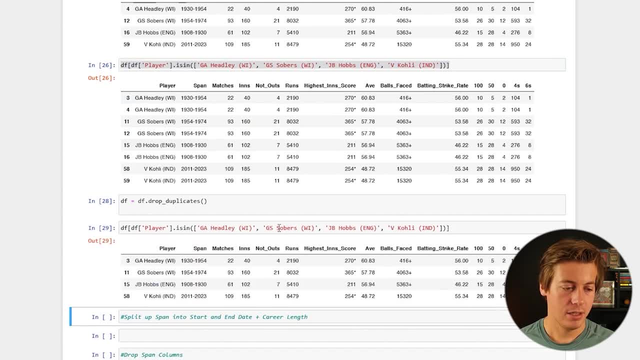 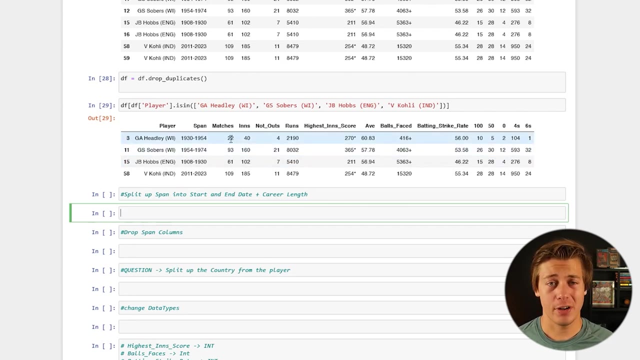 Just to show you that there's only four this time, And you can see it's been cut in half. We have the one earlier, which is eight, And this time we have four. So it is working properly. So now I would like to start manipulating some of these different columns over here. 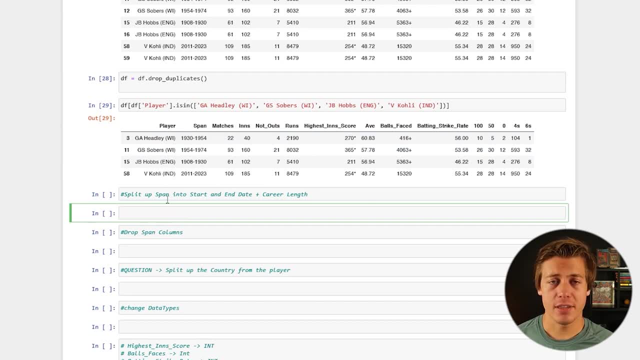 and creating new columns and series. So the first thing that I would like to do is split up the span into like a start and end date, And eventually I want to do a career length as well, But we're going to do that a little bit later. 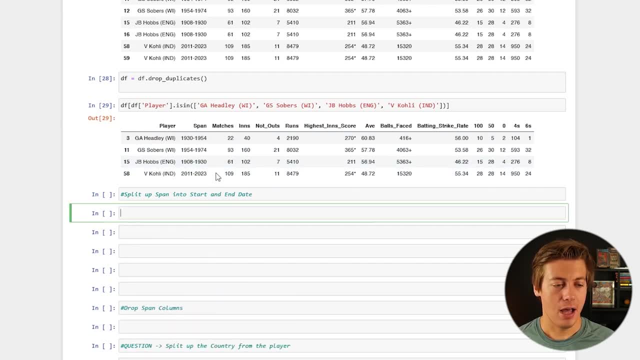 So I just deleted that. Don't worry about that for now. But I don't like the span, because if we wanted to pretty much find players that started like in 1930s or 40s or before a date, that's just not the most ideal way. 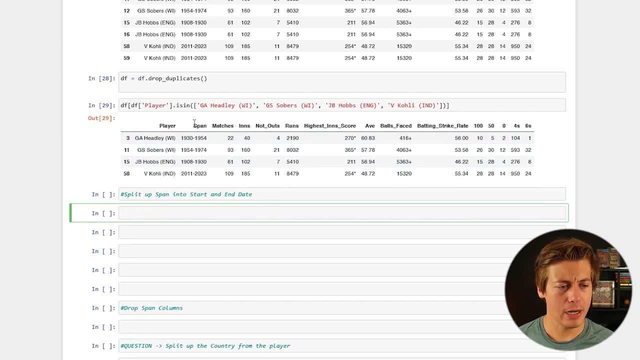 Instead we can have two new columns. So We're going to have to figure out how we can split the span, because if we just run this on here and just put over here like span right, this is what our output is going to be. 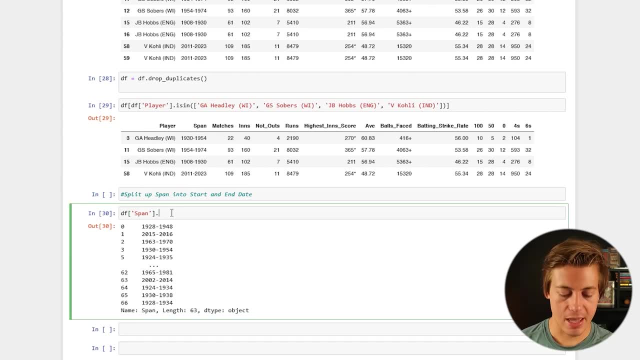 But luckily there's a pretty easy way, So we can do dot str like this for string, and we're going to do split. That's another thing. These are strings right now. They're not integers, which would be ideal for some calculations. 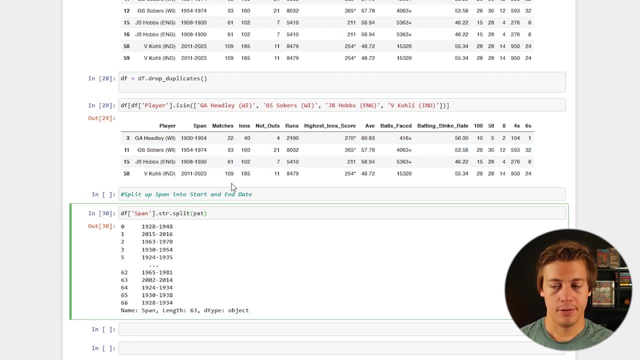 So what we can do is say Pattern like pat and then equals, and we want to split on this over here. So just put that right here, like this On the dash, And now you can see it's been split properly. right, The first part. over here we have 1928 and 1948 for Donald Breivin, the GOAT of cricket. 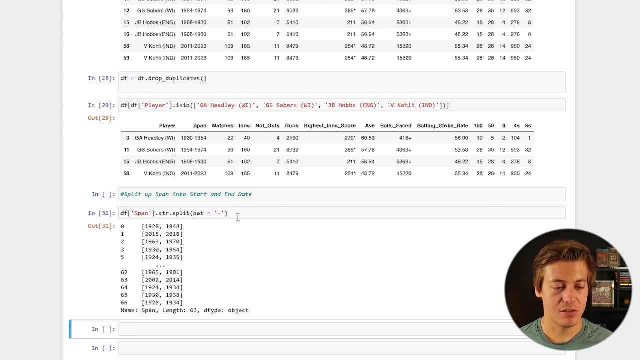 And then 2015,, 2016,, 1963, 1970.. So we know that works now, but Okay, Okay, Okay, Okay, Okay. How are we going to assign, you know, our start year or like a rookie season, and then? 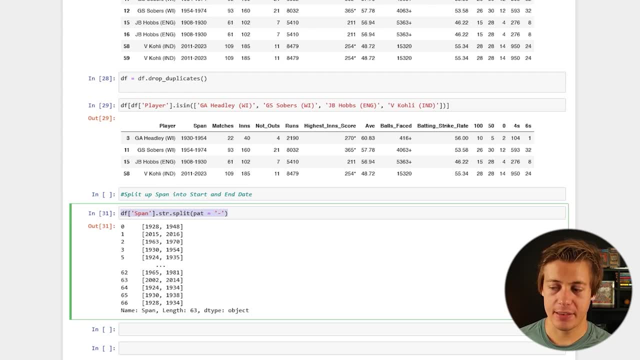 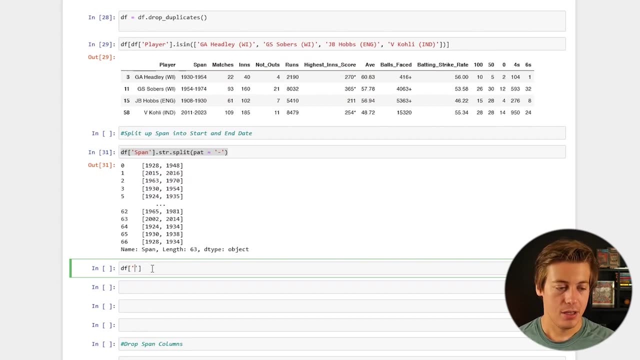 our final year. Well, let's think about that for a second. So let's say we're going to have a DF and we're going to create a new column. So let's say, like we'll have rookie year, right? So rookie, and we'll put rookie here. 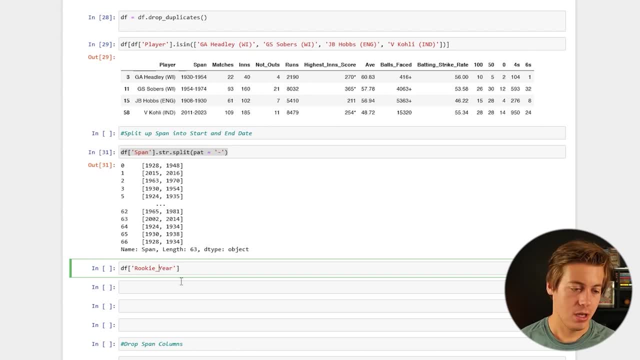 So that's the first year that someone place And we're going to say that is equal to this over here. But the Grab that first part. All we have to do is put dot STR zero. So that'll grab this side. And then if we wanted to grab the other side, it's going to be one. 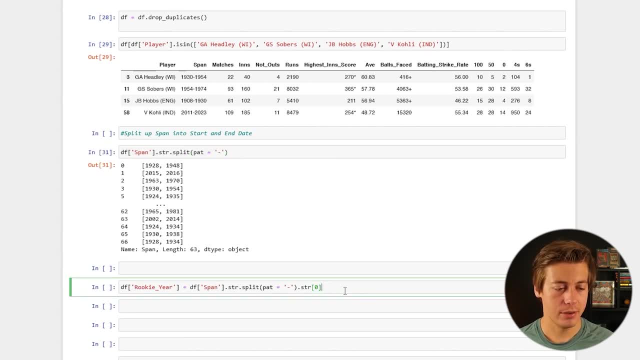 So, before I run that command, I'm just going to show you what that looks like, Just to make sure that it also works too. I don't want to have a bad data frame, but you can see zero grabs, all these on here. 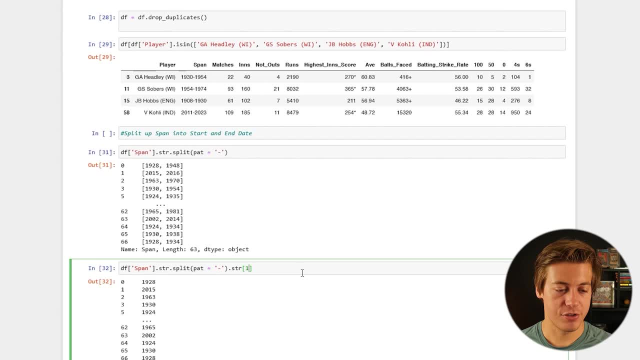 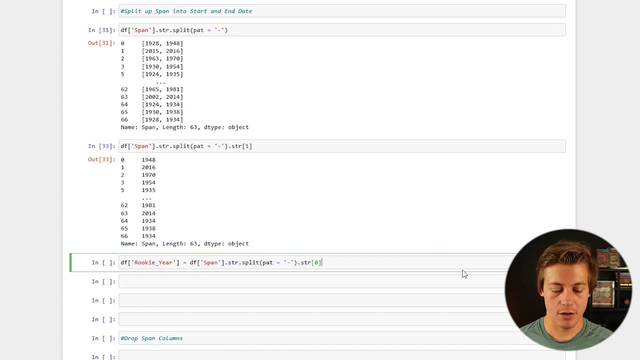 So it works properly. And then if I wanted to grab one which is going to be on the right side, Right 1948, now, So that's working properly, Let's say rookie year, Is that zero? And if I was trying to set in the copy slice, don't worry about that too much. 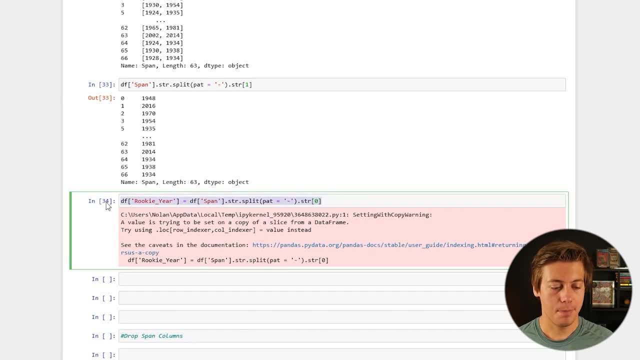 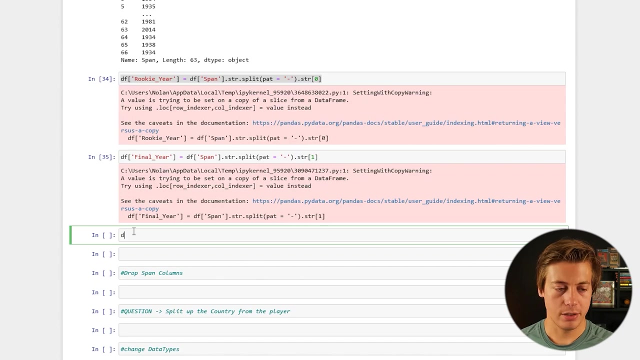 Great. And now we're going to do the same thing, but we're going to say final season or final year, It doesn't really matter, And we're going to do string one and run this again. And if we go back into our data, 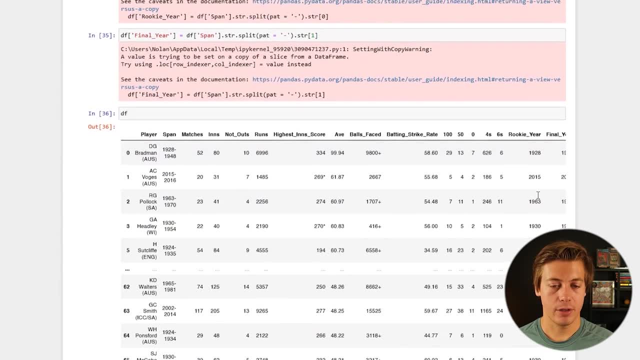 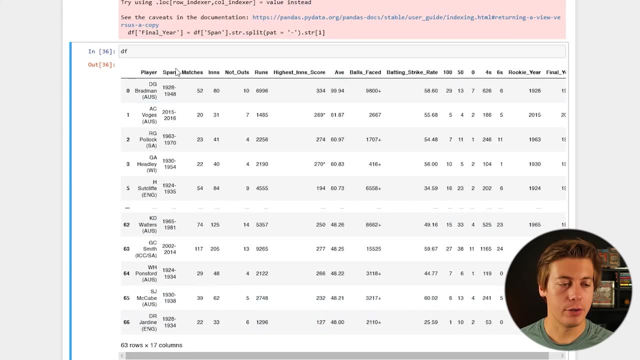 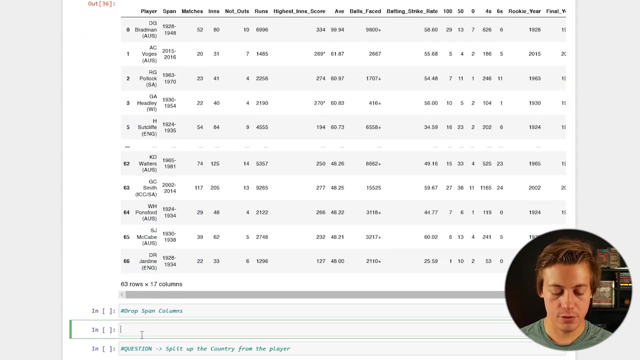 Frame. you can see, now we have rookie year and also final year over here, So this is working properly, which is really good to see, But we really have no need for this span anymore, So let's get rid of that. So to do that, all you're going to do is df, dot, drop. 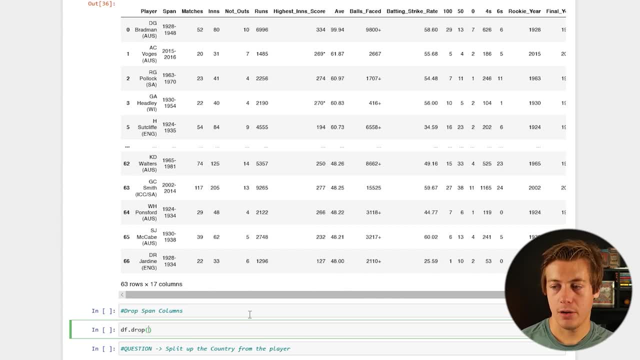 And then what we're going to do is, inside over here, we're going to put span, So span Capital S rate, because it's not lowercase, And then we have to determine what axis. So, since we want the column, it's going to be: access equals one. 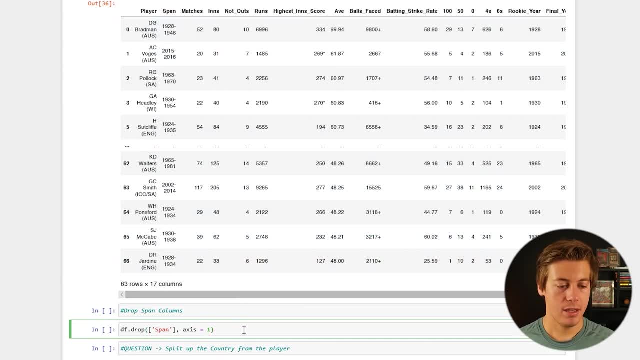 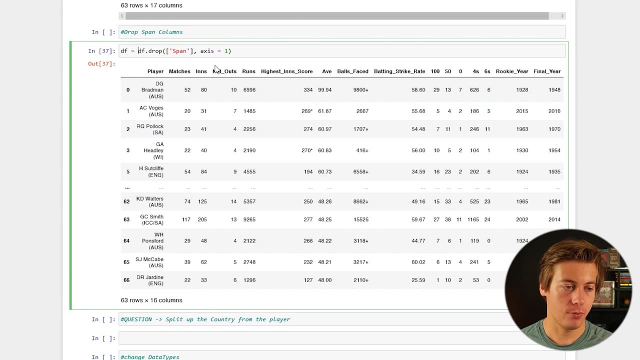 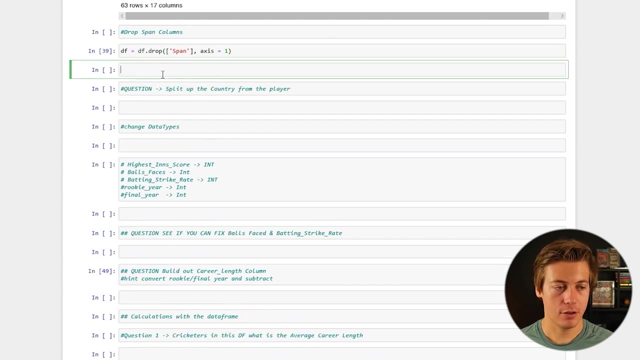 So access equals one. And then if we shift enter, you can see span is now gone And then again go back to your original data frame. So df equals df dot- drop span. And if we want to, we can go back over here: df dot head. 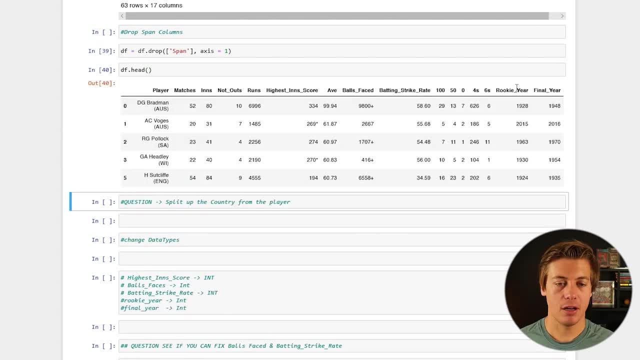 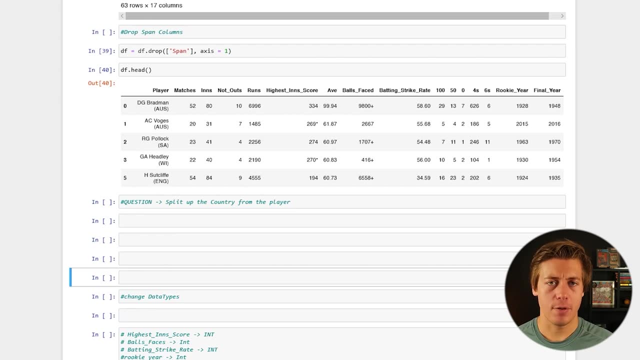 And you can see, span is now gone And we have rookie year and final year at the very end. So here's a question for you guys. There's probably a few different methods on how to fix this up, But I want to update this player. 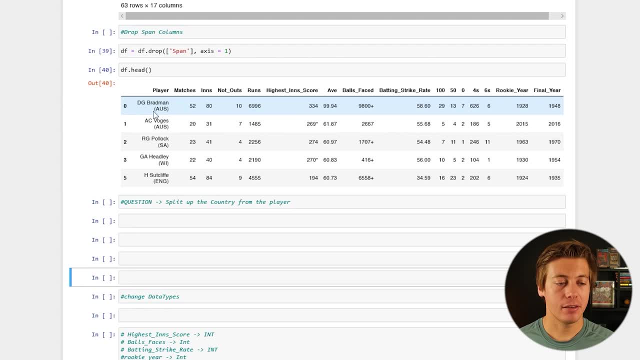 And there's a few different reasons on this. I don't like having the country code underneath on this side. Things will, if this was expanded, be over here to the right, But I just want the player name. I don't want the country and said I want to have it. 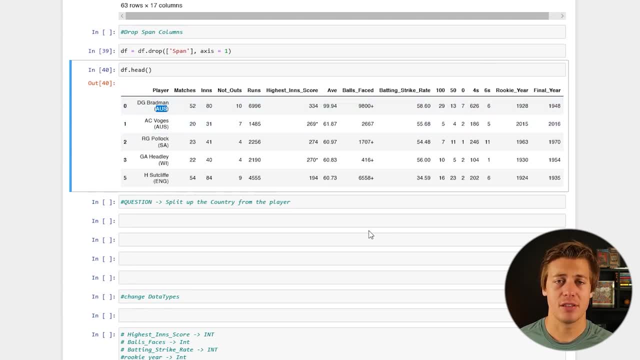 So I'm going to have another column over here for country, So that way we can run some calculations a little bit later. So if you want to pause the video, do it right now and solve this. So essentially, I want to have player, just have the player name. 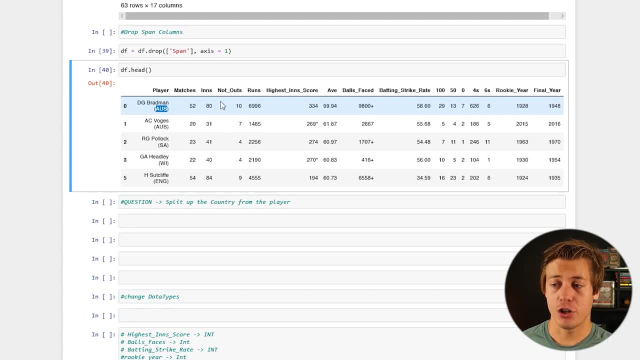 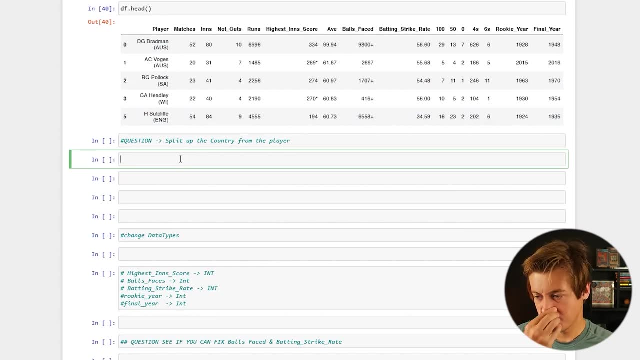 and then another column or series that says country. Otherwise, I'm going to show you a pretty similar way to like what I did over here to be able to accomplish this. Okay, So what I'm going to do first is I'm going to be lazy. 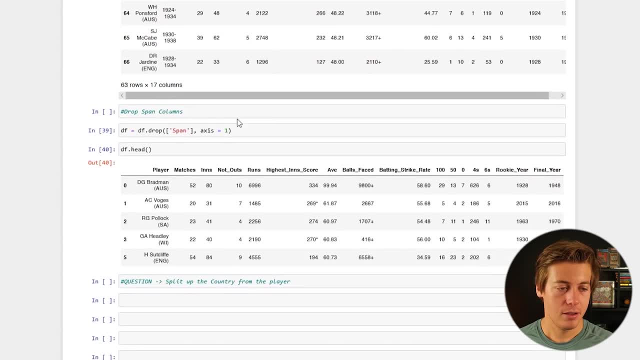 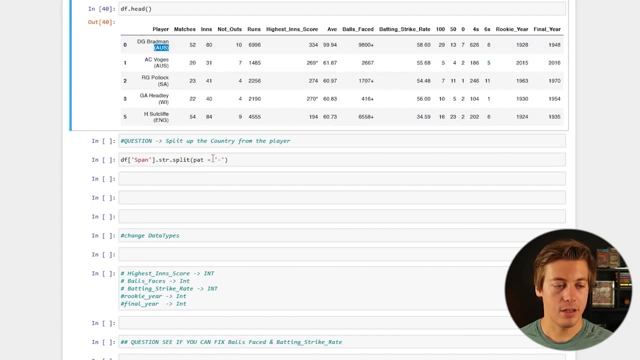 This code over here and show you exactly. So this time we're looking at this over here, So I got to change it like this, right, And I'm not going to do both sides. We're going to run this twice So you can see what happens on there. 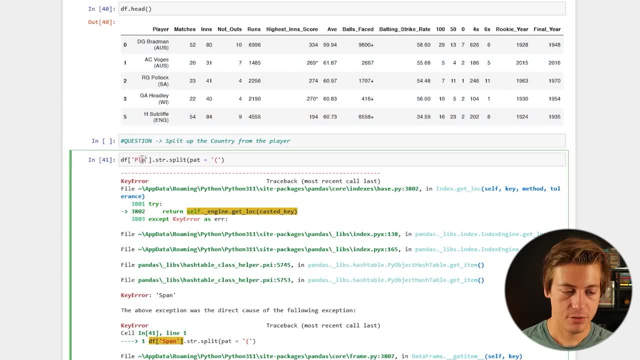 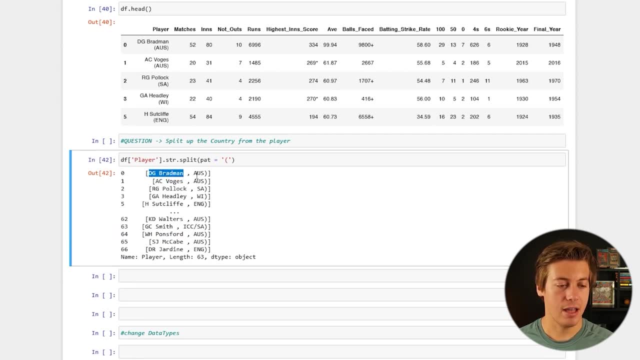 And I get an error because I meant to put player, not span. So you put player in here and then you can see: great, We have Donald Bradman. That is Working correctly on the left. The right is not working only yet, but that's okay. 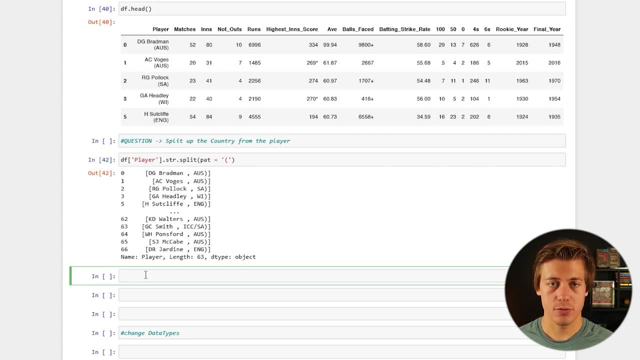 So what we're going to do on this side of things is, first, we're going to name the country, So we're going to say DF country, and that's going to be equal to- and I'm just going to copy this here: 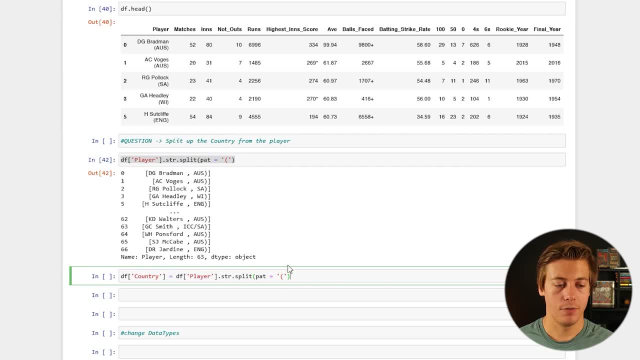 And, like last time, one is going to put over here to the right. So I'm going to just say STR one and We run that and we just can do the F country like this. right, We have this going on and we can fix that a little bit better. 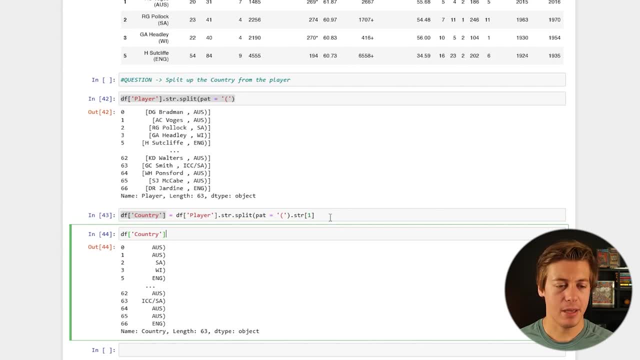 So all we need to do again it's kind of like the same command as earlier, So I'll show you how that works. So we can just do DF country, like this, and we're going to do that string split, And this time we're going to do the right side. 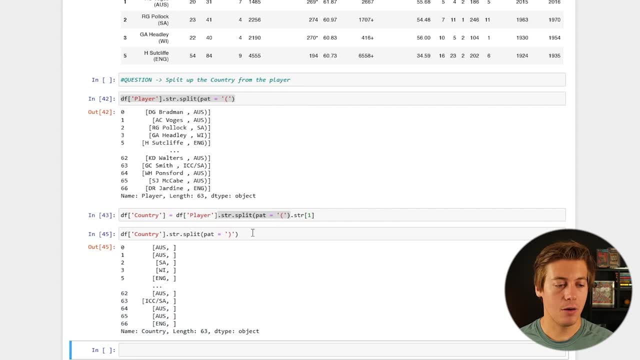 Since we did the left last time And you can see, now we just want to grab the left. So we can just say that's string zero, Grab string zero. And I'm just going to say that country equals dots. And then if we run the F country, 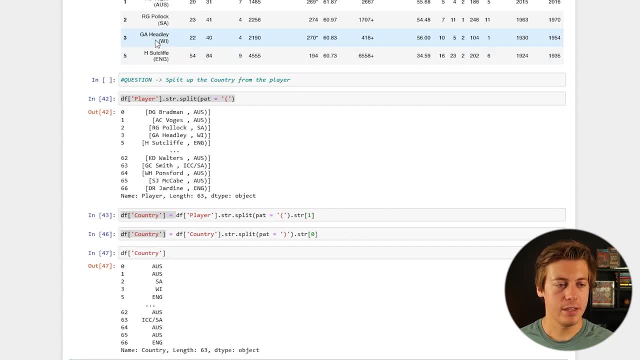 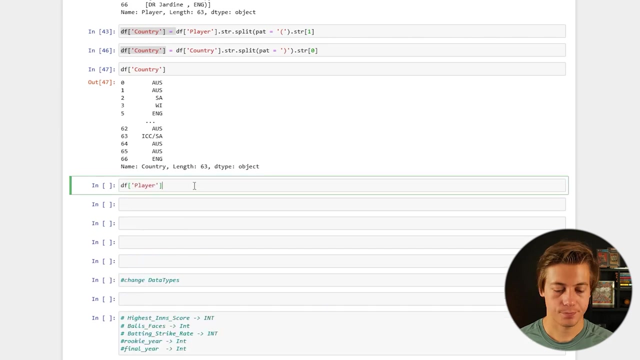 Great, We have that working, so it's good. But we still need to fix the player on here, because if we run, if we run player, it's still going to show the country code. Yeah, And I'm just going to put a few more here, right? 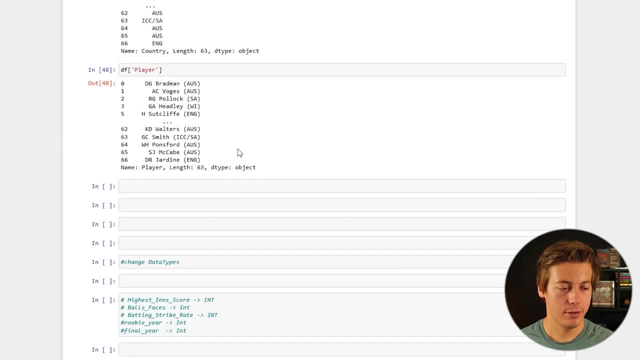 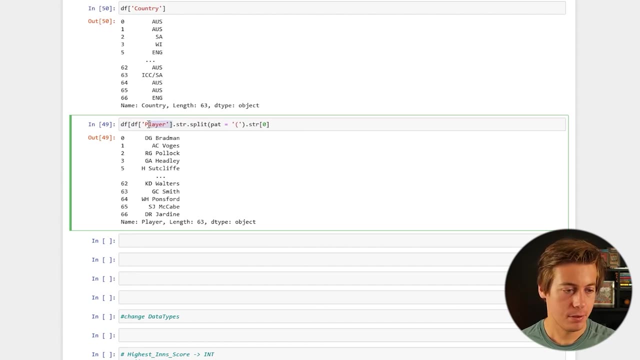 We still see the country, but I kind of show you how to do it a little bit earlier. So if we go like this, what we have to do now is assign it back to DF player. So DF player, like that- and I'm just going to copy it instead of typing it all out- equals this: 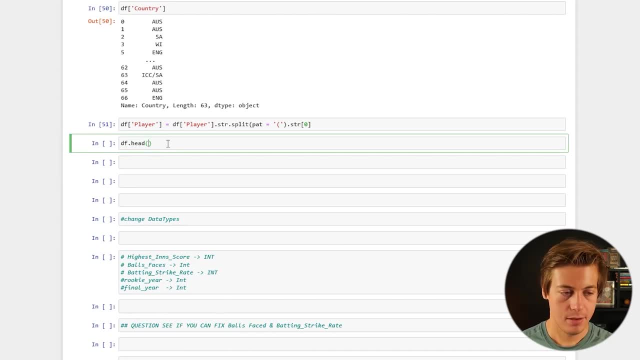 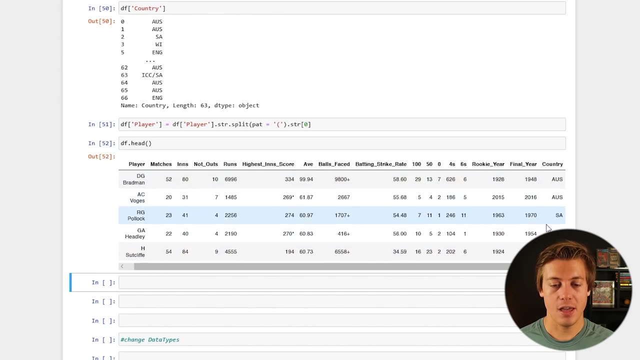 If we just run our data frame again- So DF, the head that's, you can see we have player which the country code is gone, But all the way at the very end we do have the country, So working great right now. 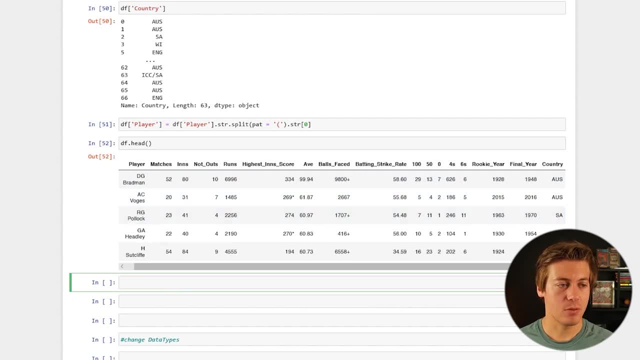 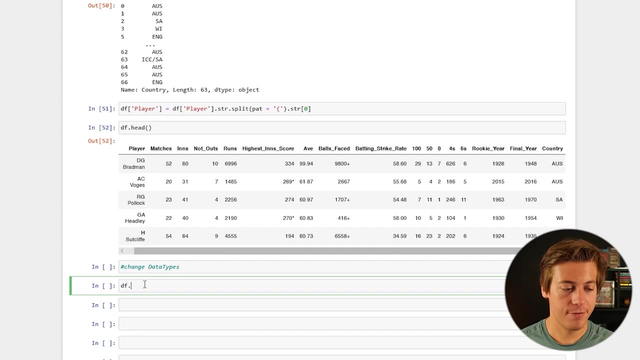 This data is already looking way cleaner. But next we need to fix up these data types, because they're not all going to be correct. So all you have to do to see the data types on here is put DF, dot, D types like this, And then, if we run that, 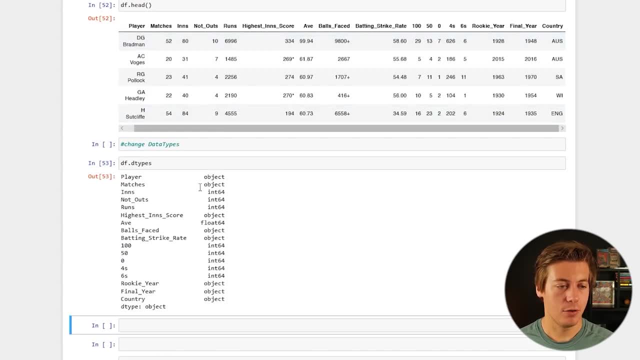 You can see, player is an object. Matches is also an object, which I think this should be an int, not that, So we might have to fix that. We have some integers over here, which is good. Highest inning score is an object also. 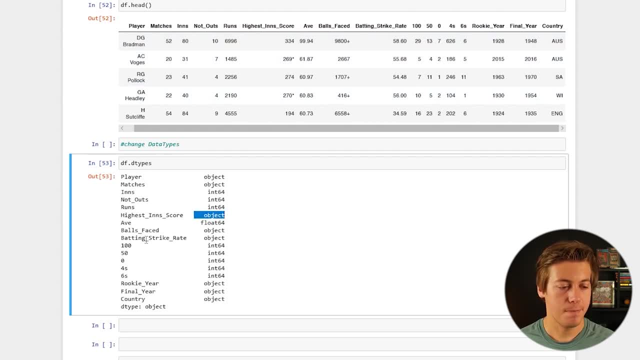 So that should be an int. Then balls face in batting strike rate. So batting strike rate should probably be a float, not an object. Balls face, That's a singular number, but that should be an int. But you can see that. 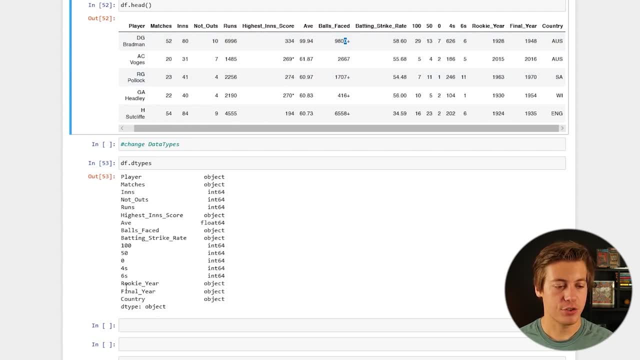 We have some issues with that. plus, over there, All these are ints, which is good. Rookie year, final year, should both be ints and then country. It's fine like that. So we have some work to do. right, We got to figure out why it's not working properly. 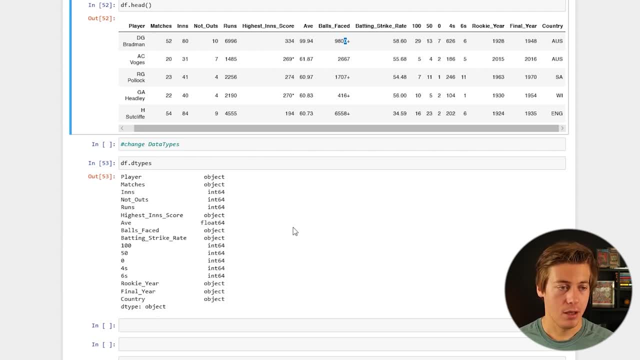 So let's take a look at one example over here. So the first one I want to take a look at, since it's pretty obvious, is this: highest in score. So that's this one over here. It says it's an object. 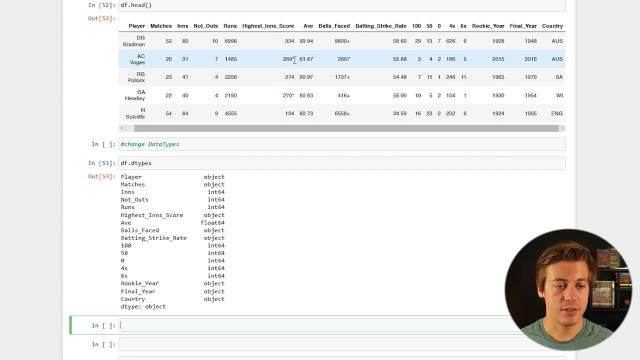 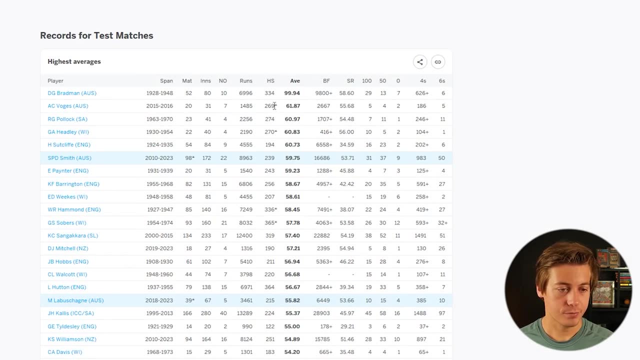 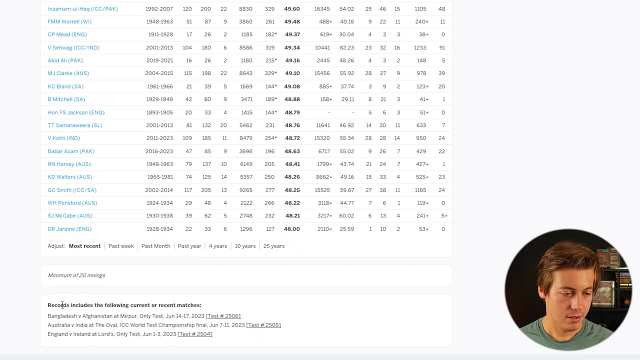 So The reason why it's an object is if you see this star, So the data for these stars, if you go back over here just to take a look, you have a star right there, multiple stars over here, And I'm trying to see why it mentioned that there's a star in there, but it doesn't say 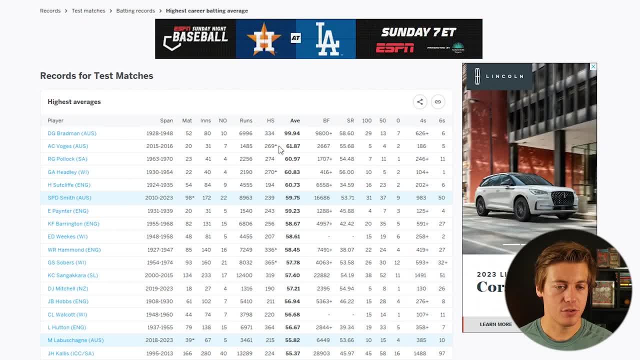 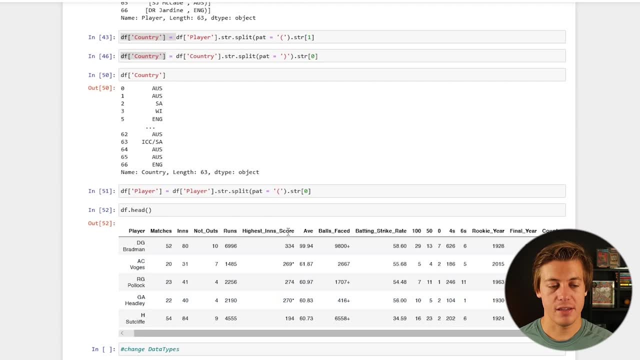 anything why that star is in there, So I'm just going to remove it. So if we go back over here, let's go back to what we did. also like this String split. So currently this does work as a string, but we can fix that. 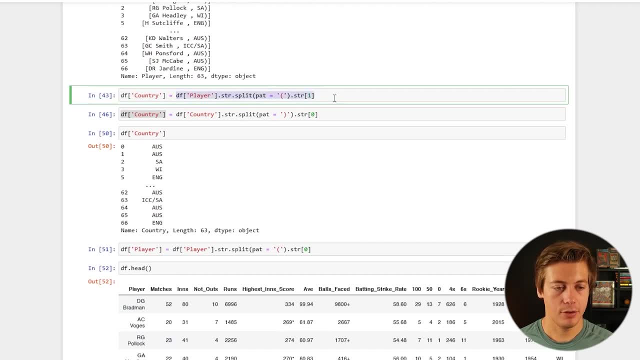 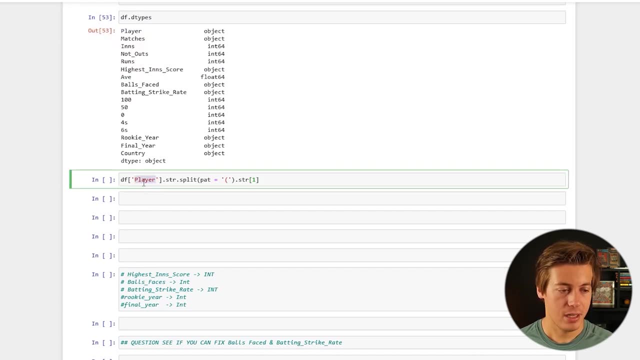 So Copy your code on here And what we're going to do is grab this highest in score right And in a string split, And this time we're just going to put a start right And put it like this: Now, this doesn't look like it's working properly because it has that comma. 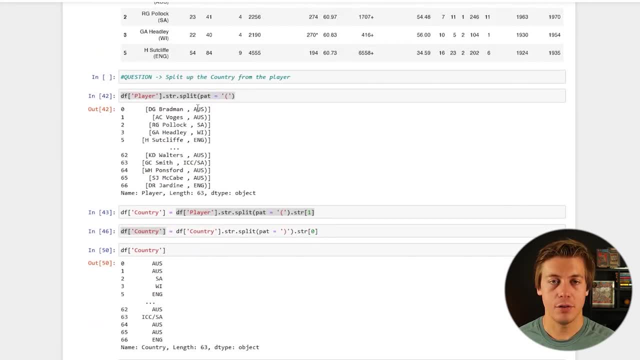 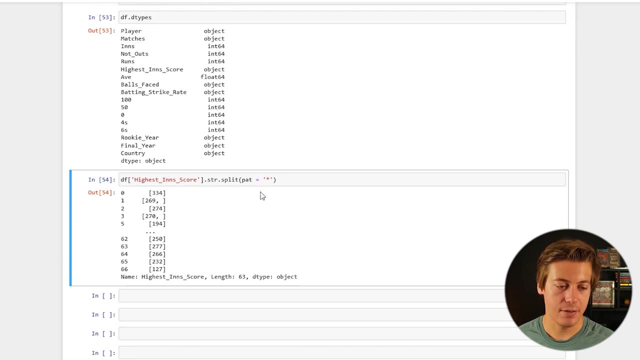 But if you remember from before I had the common Comma is just going to show you where it's splitting at in. the second part is to the right And since we are splitting on that star, it's just going to have a blank on that side of. 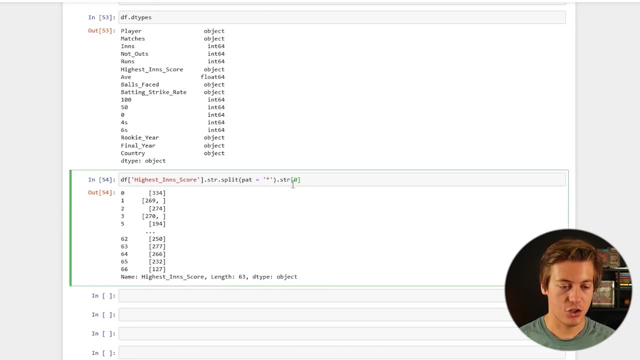 things. So if we put the STR zero, so like this, it should show everything properly. So just run that for a second and you can see that star is now gone. So again, kind of like earlier, let's just assign it to itself. 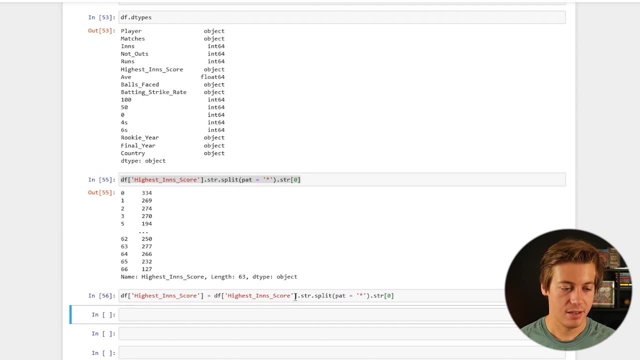 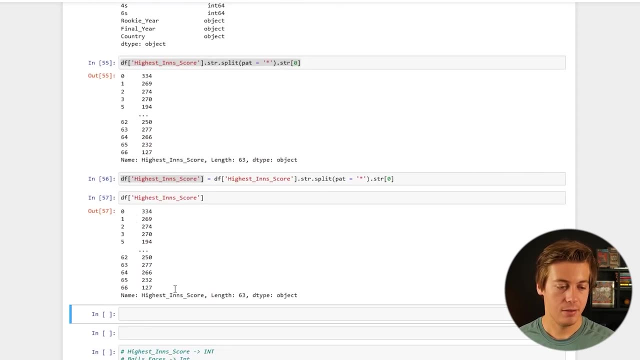 So we just put that over here equals that, And now this is going to be working Properly. We we can just copy and paste this here. You can see it's gone right. We had it originally at two 69, but two 69 is like that. 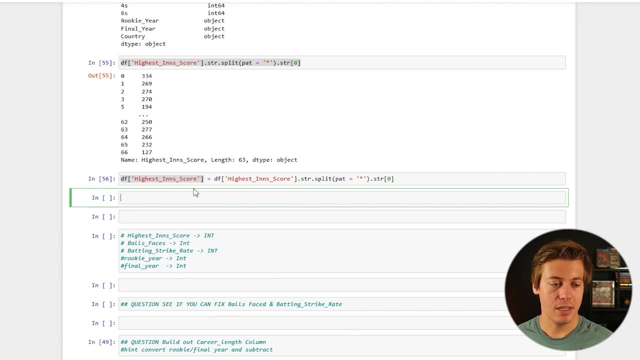 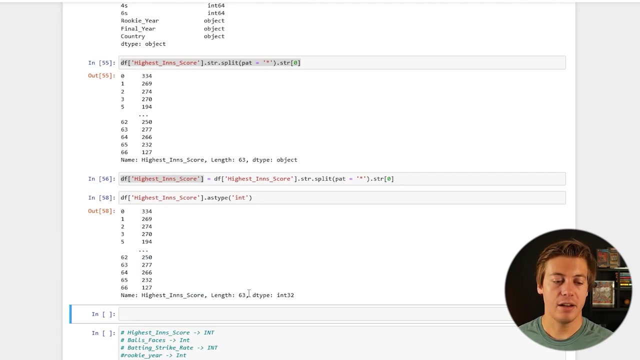 So it's cool. Now we need to specifically say that it's going to be an integer. So the way you can do that is dot as type like this and just call an int in here, right? So int on here And you can see down here. 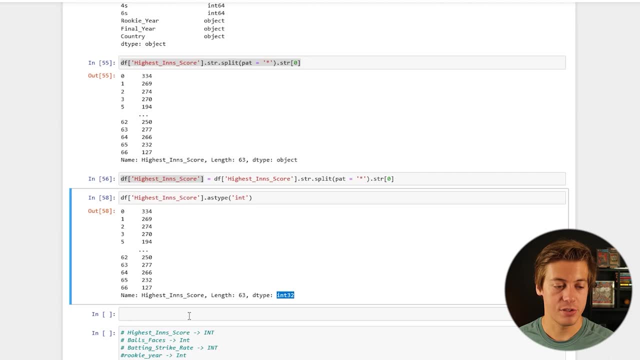 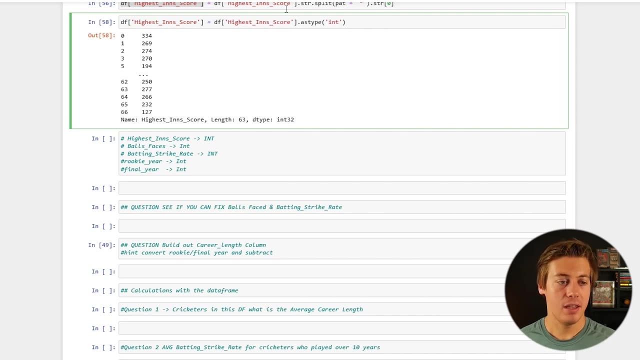 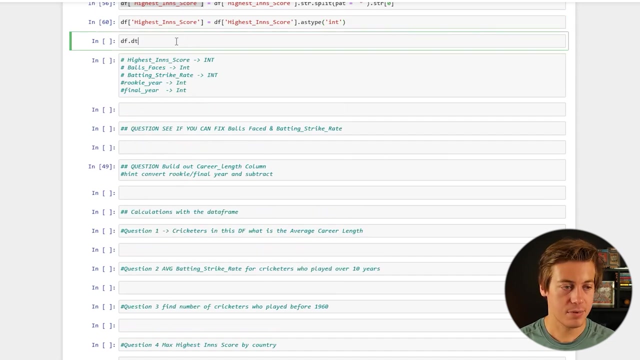 It says D type is int 32 now instead of object, where it was before. So now we just have to assign it once again back to where it was. So ending score equals that That's going to be gone now. Just put the F dot D types. 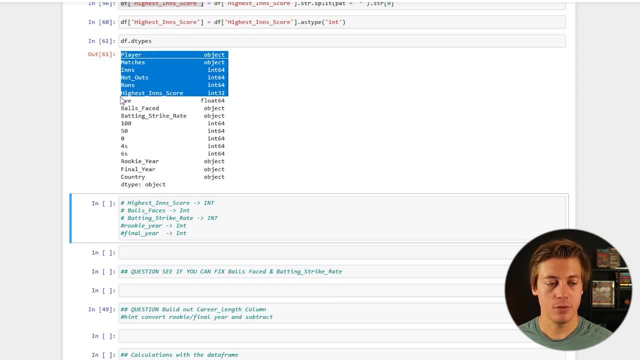 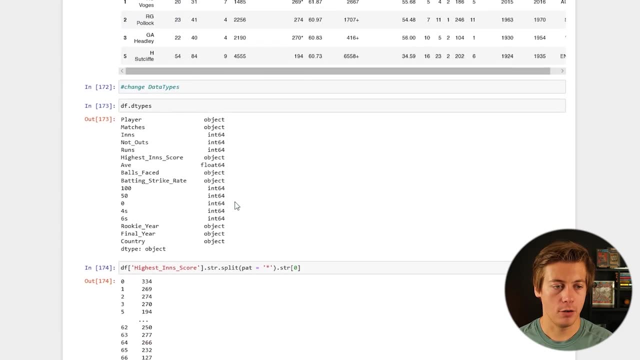 And you can see: highest ending scores now is an int 32.. Okay, So question for you guys: let's see if you can fix either rookie year And final year. So if you remember from earlier, um, we built out those new columns. 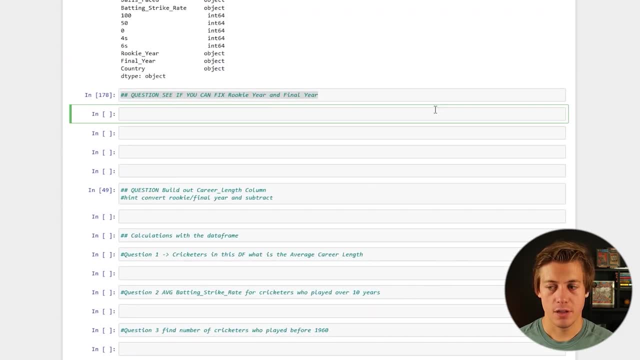 rookie year and first year, So see if you can convert those. I'm actually going to show you a pretty cool shortcut on how to do that. Um, so all I have to do is D, F equals the F dot as type, like this and inside over here: 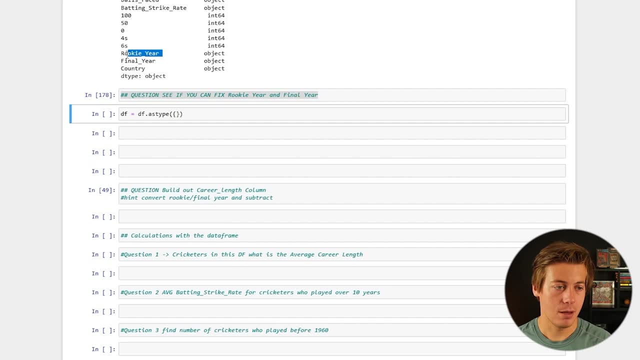 what we're going to do is build out a list. Okay, So I'm just going to go ahead and do that. Okay, So I'm just going to say rookie year, and then I can say colon. We're going to say this is int, and we can do the same thing, uh, with final year. 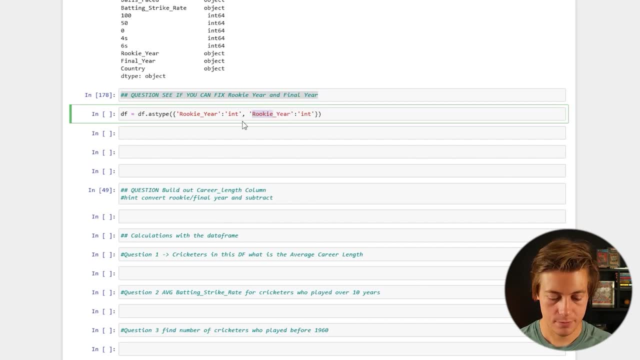 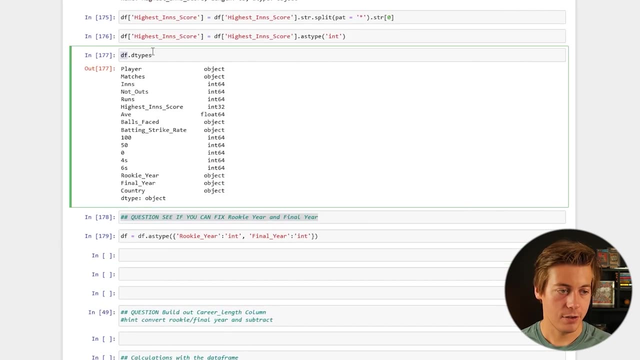 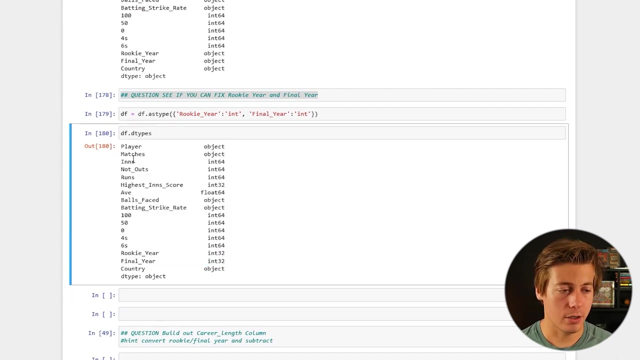 that over here final year. And then, if we just run the data frame again, uh, for D, F, dot D types, you can see that both of these are in. So we have three more that we need to work on now. So we still have matches. 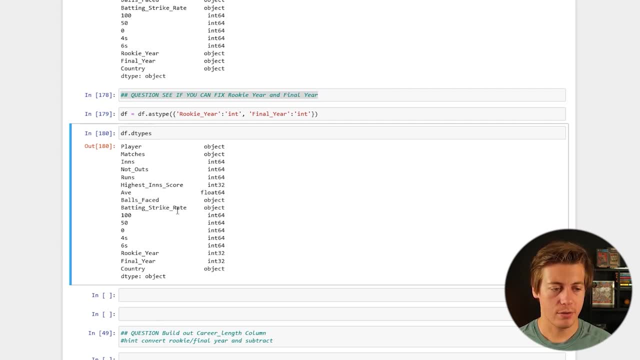 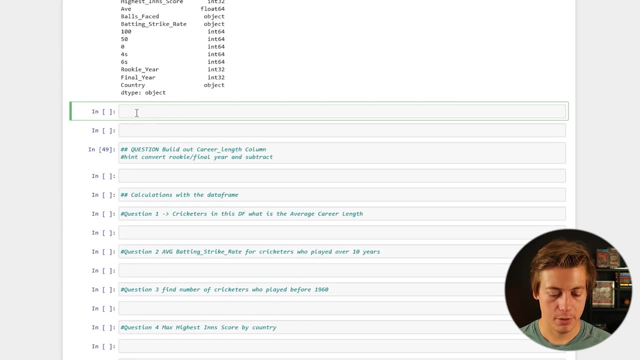 Uh, we still have balls faced and then we have batting strike rate. So if we just take a look real quick at batting strike rate- So I'm just going to put the F the head, um, batting strike rate needs to be a float. 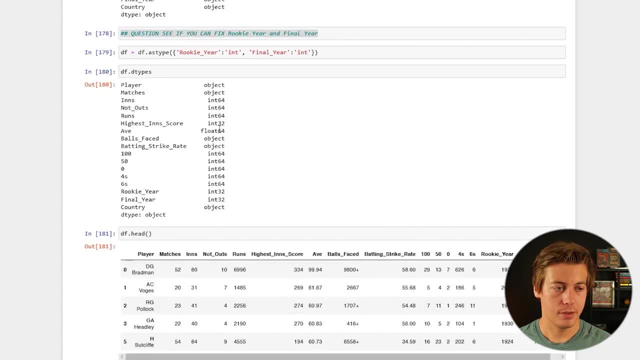 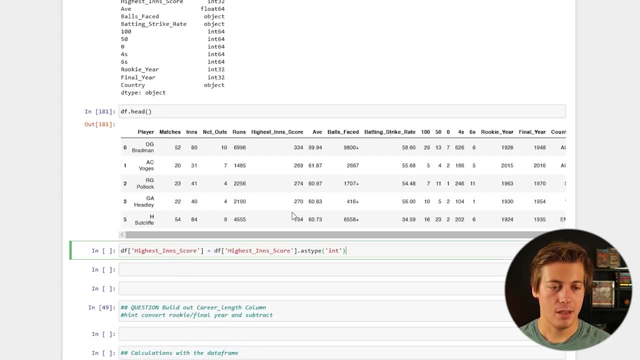 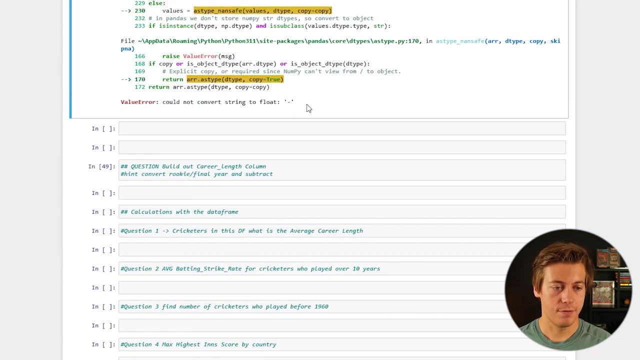 So a little bit different. Um, so again, we can just kind of do: Okay, Just copy this over here and grab the batting strike rates, That's, and then we're just going to name all this as a float and does not work, as this could not convert string to float. 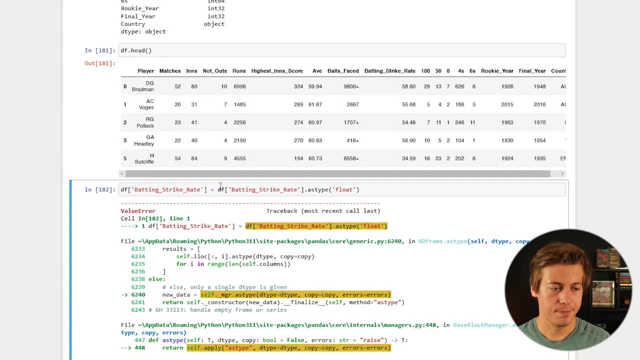 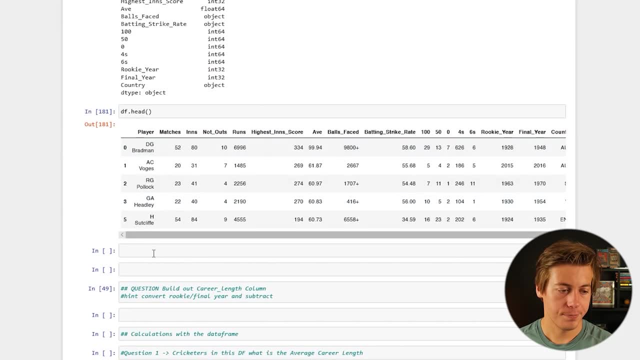 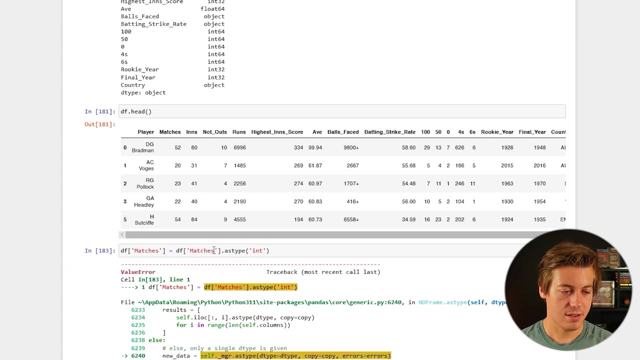 So we'll have to take a look at that a little bit later. So let's still convert matches. So like this right, Just copy this one over here. Okay, Okay, Okay, Okay, Okay, I'll put matches. matches as type int. 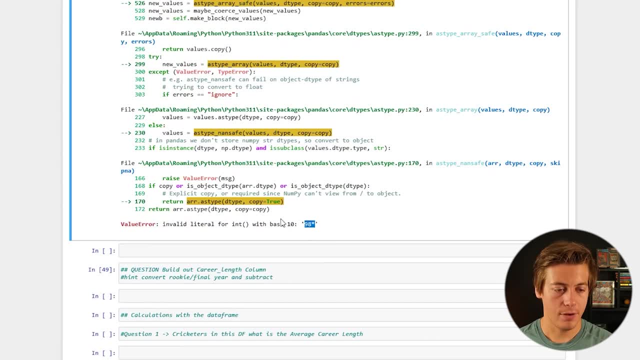 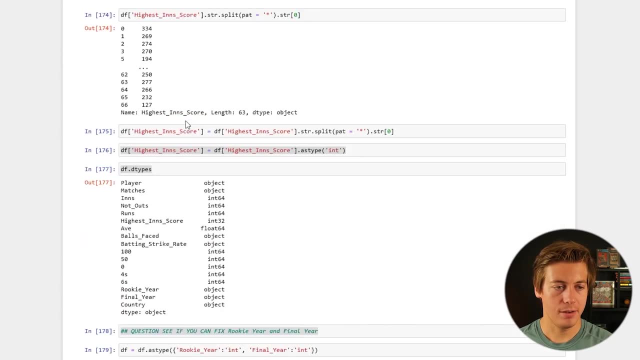 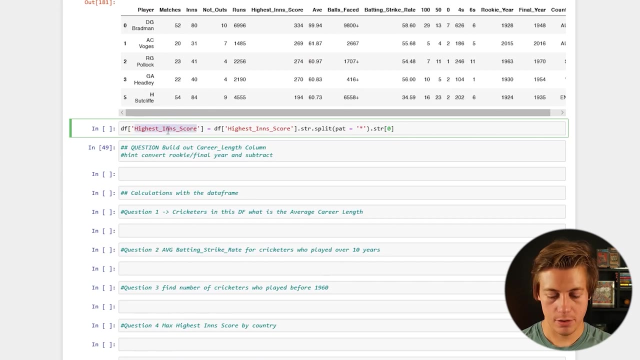 And we have an issue- 98 star. So we haven't got rid of everything with the stars yet or like kind of weird formatting. but that shouldn't be too hard. We can just copy this on here for highest innings And we're going to do just matches, right? 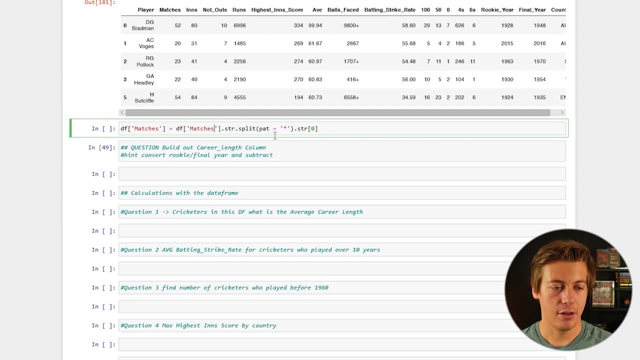 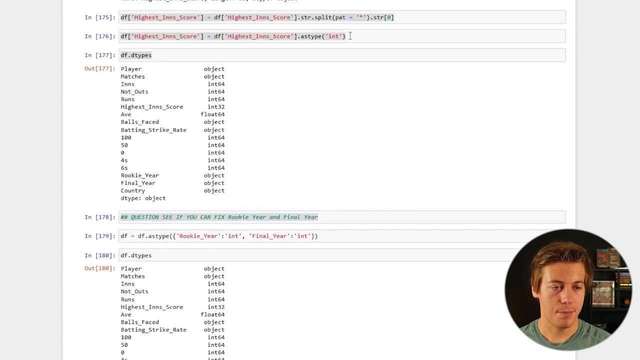 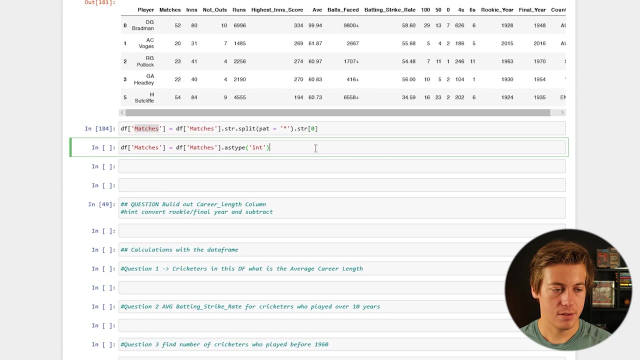 Okay, So we're going to do just matches. So we're going to do just matches. That'll grab the left side of it, And then we build out a few other lines. Let's copy this over here And it should fix matches now. 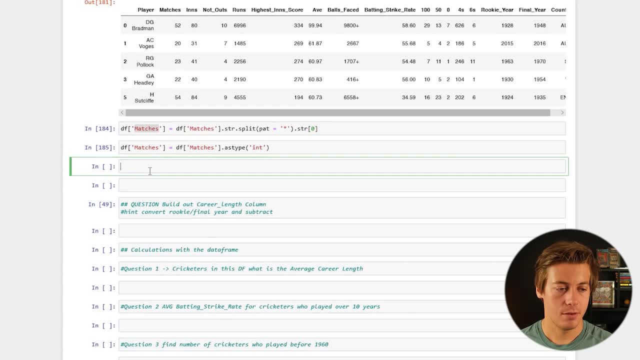 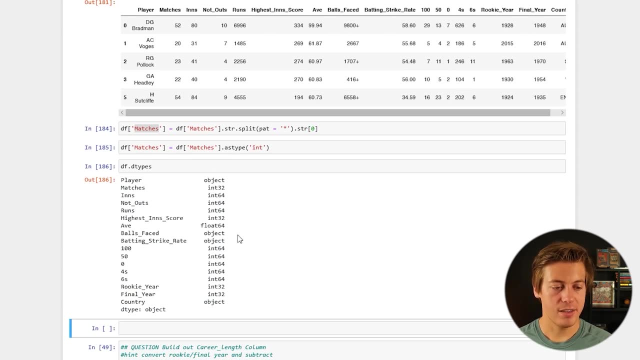 So if we run the F, dot, D types, so object for player right, That's fine of all the ends over here. A ball space is still going to be a ball space. It's still an object. batting Strike rate is still an object. 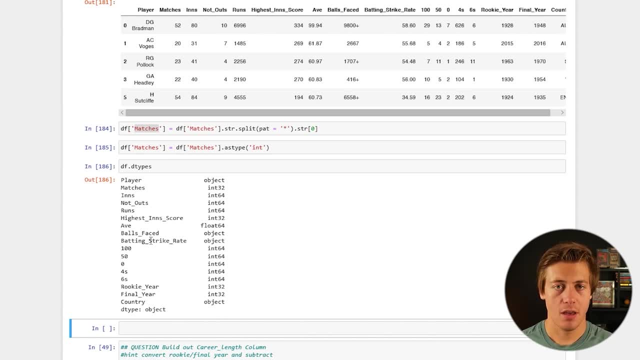 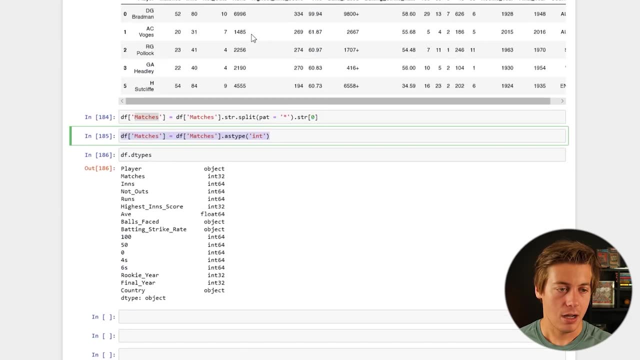 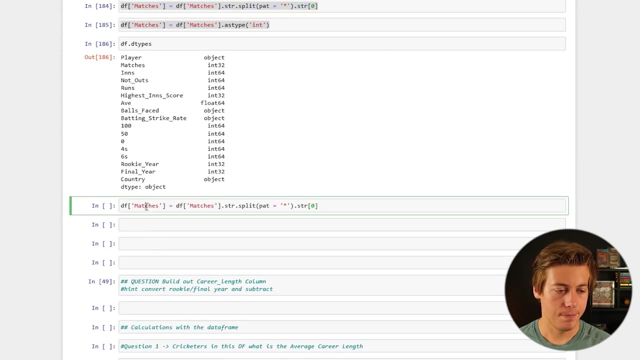 And then we have integers over here besides country, So we still need to fix all space and also batting, It's true. So for balls face, let's see we have this plus icon over here, So let's split that out. So just grab that over here like this: 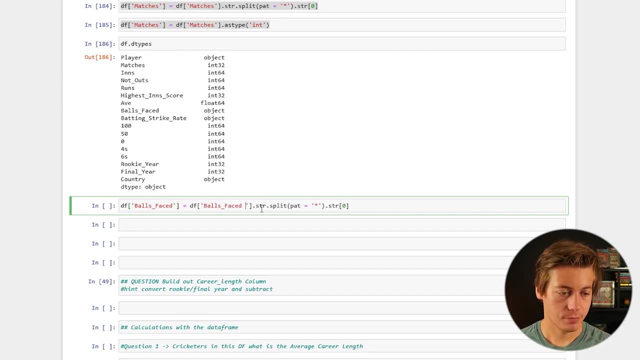 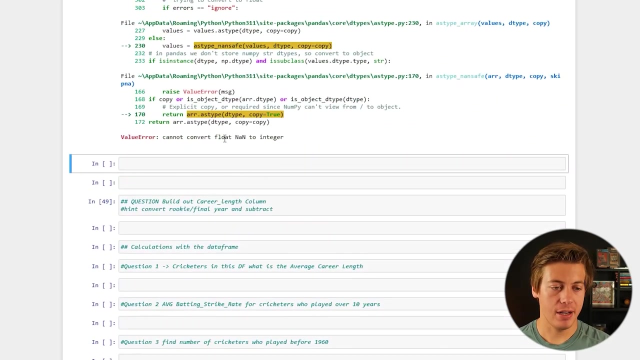 spaced. Okay, And we're going to put a plus icon this time. So that should solve that If we just copy this and we're having an issue. So this could not convert float NAN to integer And I thought we converted all the NANs. 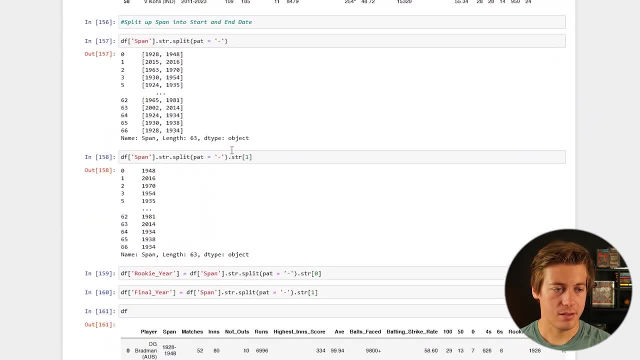 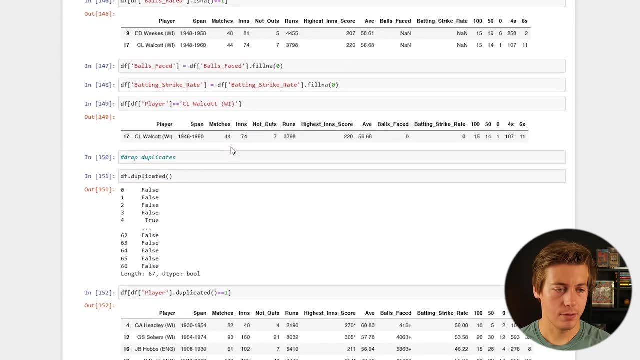 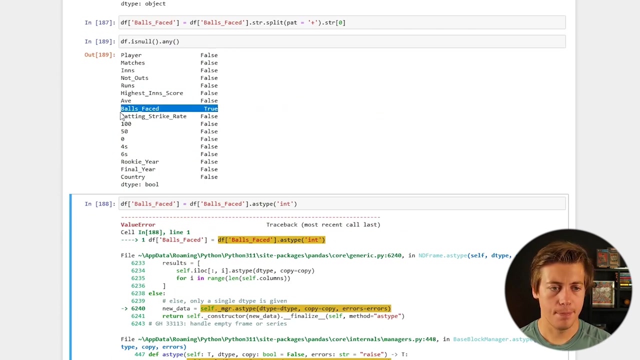 Let's just go back over here and see why that's the case. So if you remember from earlier, with our code we have it right over here. So let's see what's going on. So balls face does have a null still, which might've happened when we were doing this string split. 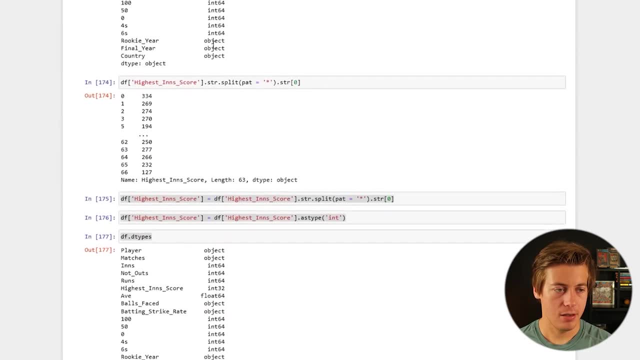 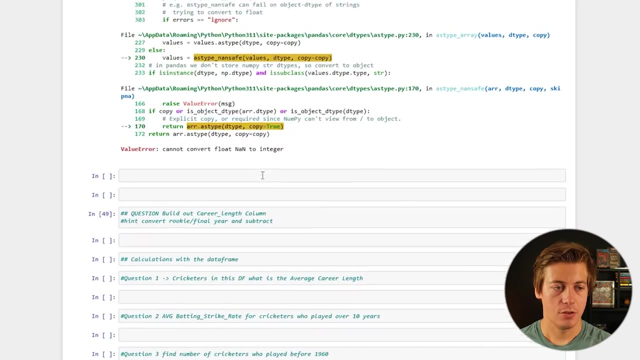 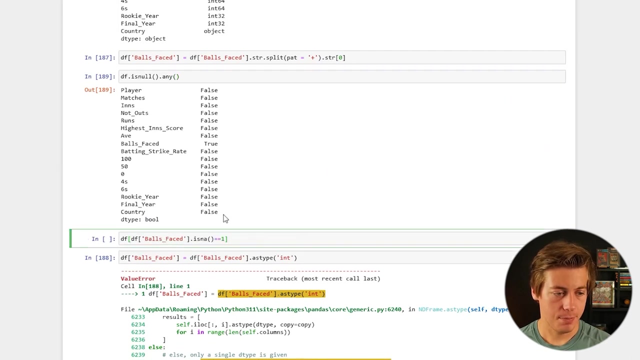 So I'm just going to copy this and, honestly, it might just be best that we drop those rows. We get some issues still. So we're just going to copy the same code we wrote earlier and see what's going on right, Because we're solving issues with balls face. 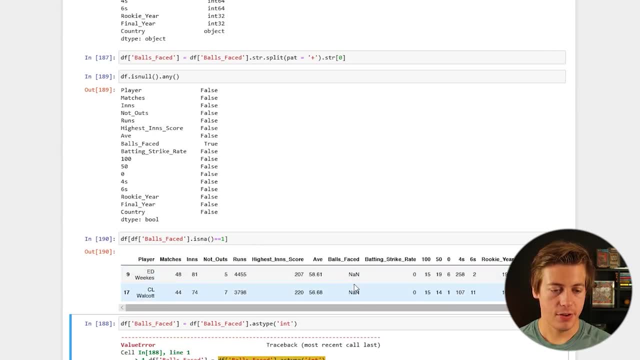 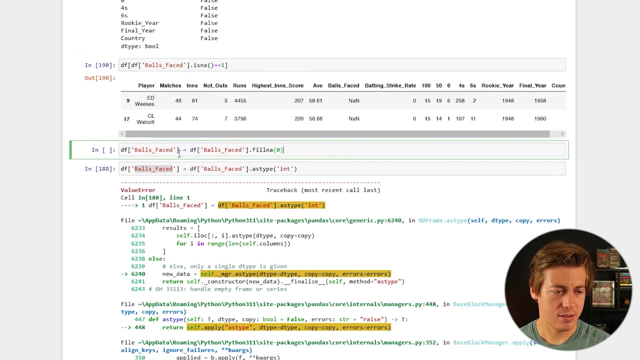 And it looks like balls face is an NAN again. So I thought we set that to a zero. Not sure why that's still happening, right, Okay, Okay. So it could be from this, but so let's try this We're going to say again, to fill NA as zero. 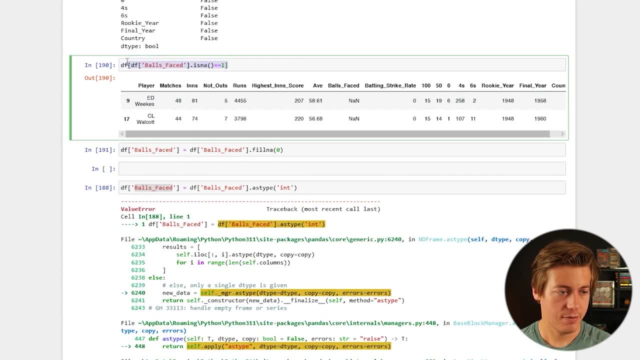 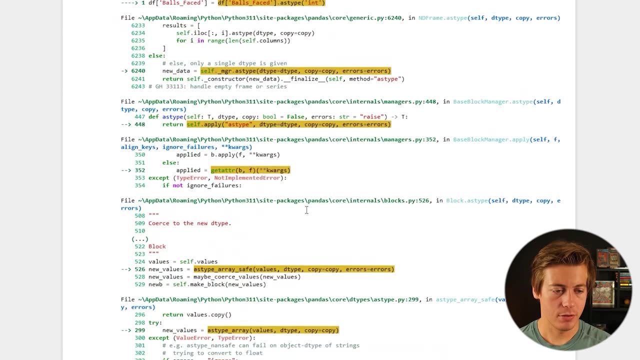 So I put another line and we're going to just see if this still exists. and there's none in there. but we're still getting an error. It says invalid, literal. Ugh, I don't know, I don't know, I don't know. 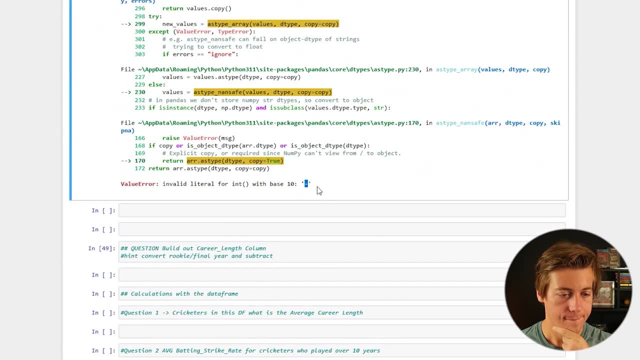 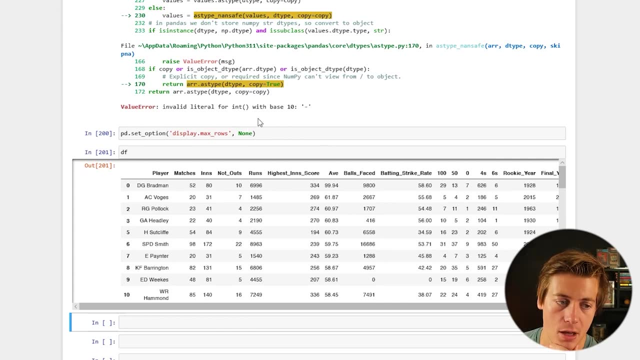 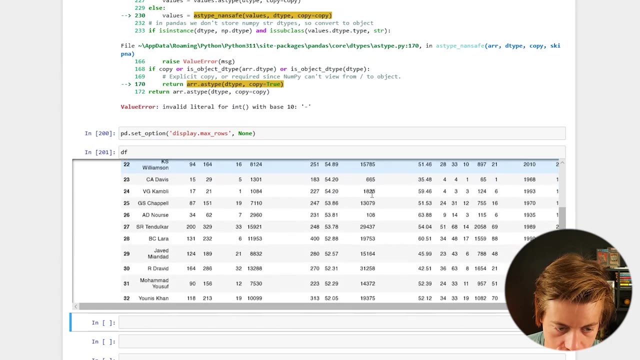 So we're still having errors. So I put a PD dot set option: display max rows: none. I'm going to take a look and see why we're getting an error. So we're going to look at balls face. So we have this on here and it looks like we have all integers. 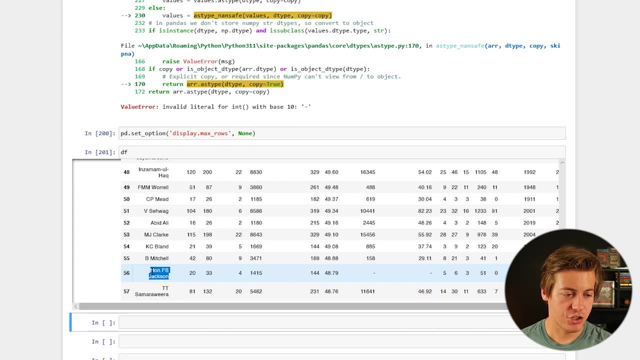 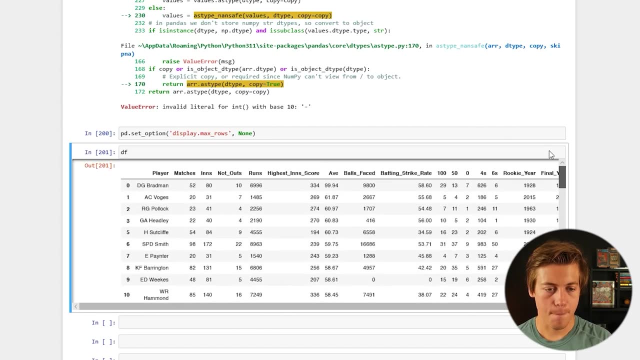 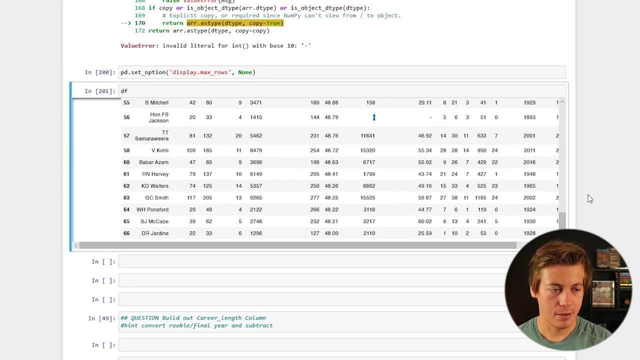 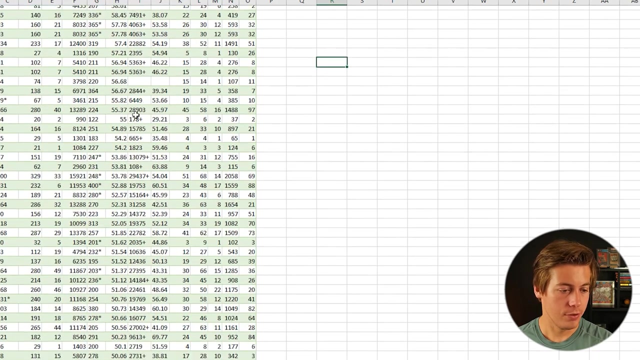 Oh, here we go. So, FS Jackson, we have this going on And then you can see also, we have that for batting strike rate. Did we miss that earlier or how did that happen? You know what happened? Um, I think, when we're in an Excel sheet and we remove those, we forgot FS Jackson. 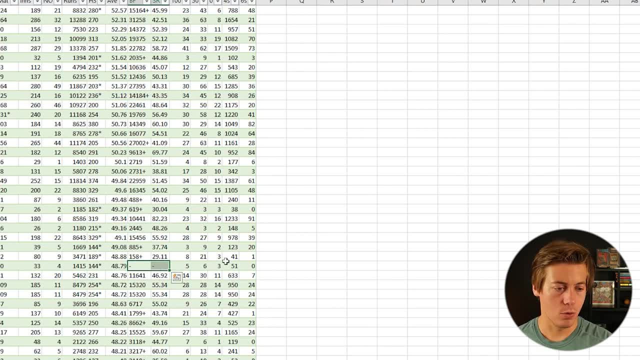 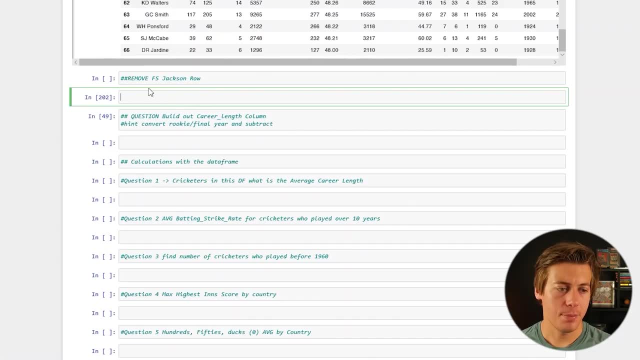 So you can see, remove that. So let's remove that. uh, row And um, that is why we've been having so many issues, man. So now we're going to drop this FS Jackson. So all you have to do is df, dot, drop and then it is number 56.. 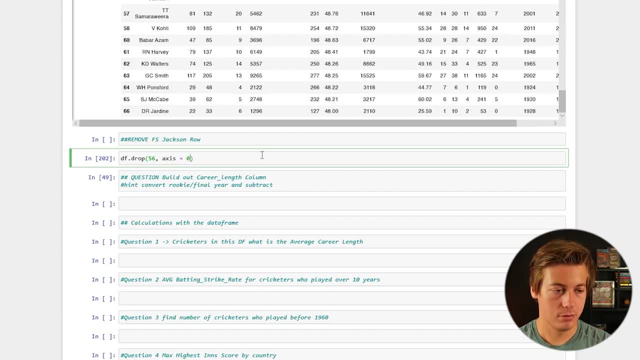 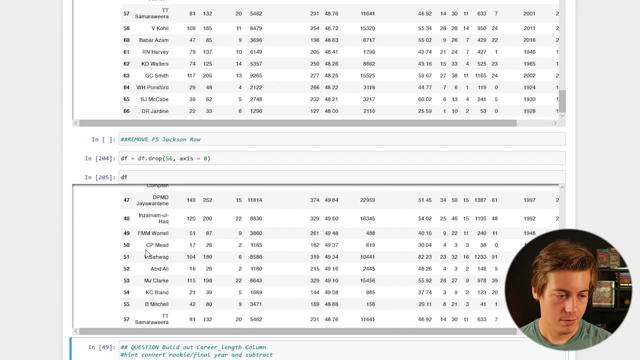 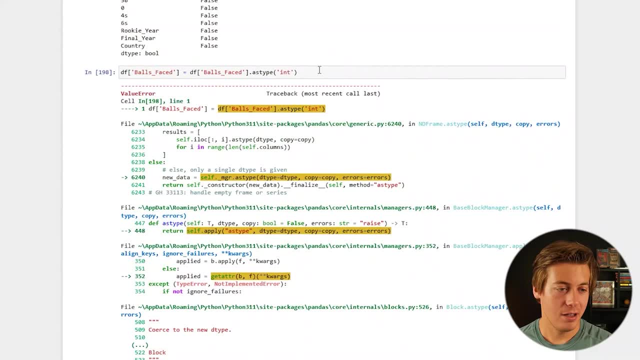 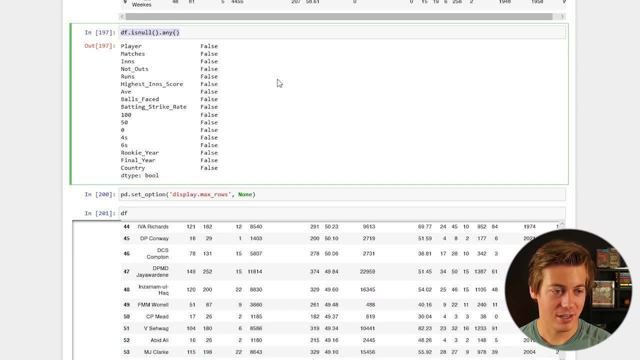 Okay. Okay, It's nice to see that You can see 56 is gone. So now the nightmare of getting these fixed should be done. So let's just go back and see. um well, first check if we have any other reasonals right. 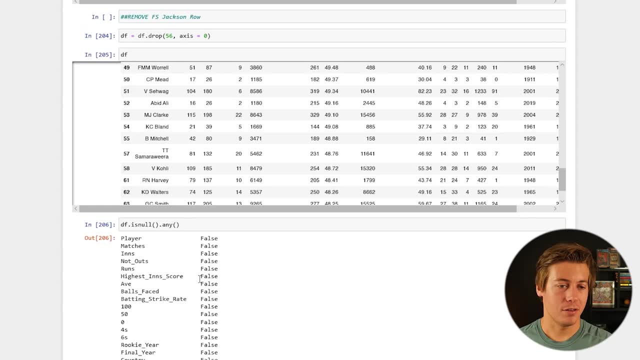 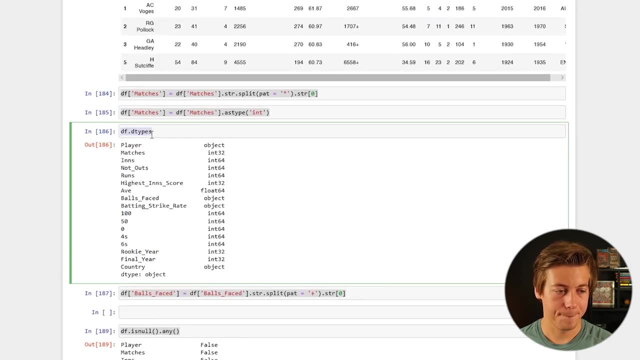 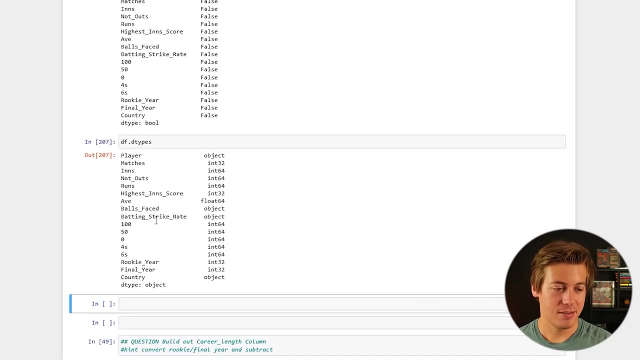 So first, all false, Okay, And we already see this over here, which is good. So now we'll just fix these last two right. And we had the df type, which was right here. Run that again and um, false face in batting strike record. so let's just copy our code from earlier. 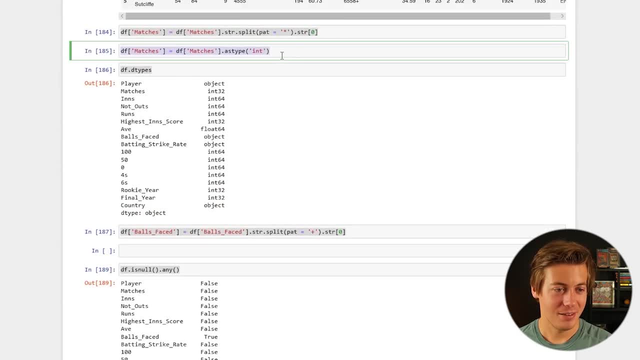 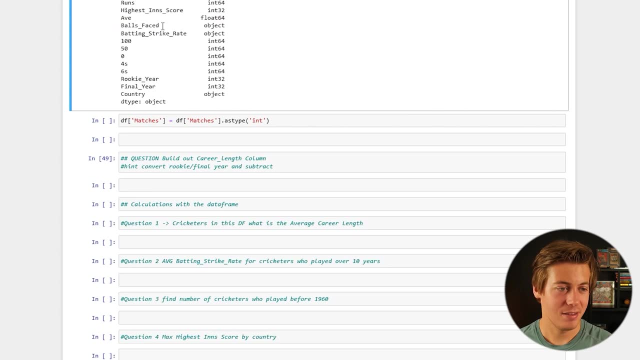 man. uh, small mistake goes a long way, right, so false face. this needs to be an int. let's grab that. this should work perfect now. and it does right and um, we'll do the batting strike rate as float and check that out. that worked too. let's run this one more time. dfd types. 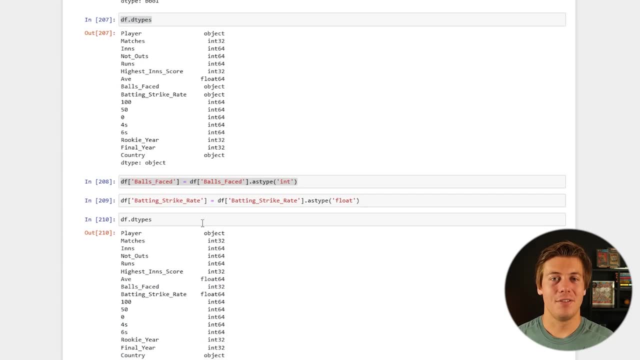 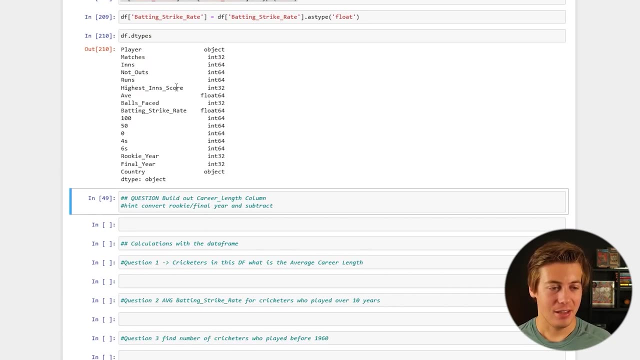 and all of the fee types are working properly, so now we can actually answer some of these questions. before that, though, um, we want to do one last thing, so find the career length. so all i'm going to do on this one is df career length, and that's going to be equal to df final year, df final. 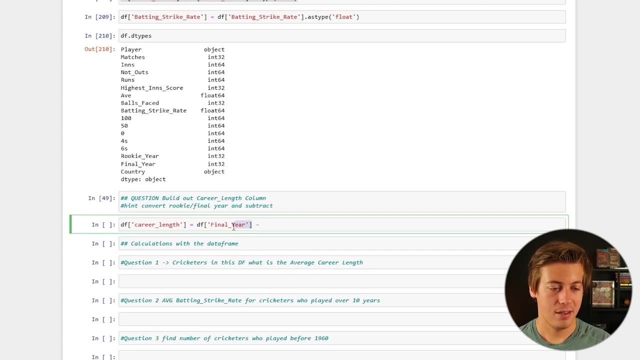 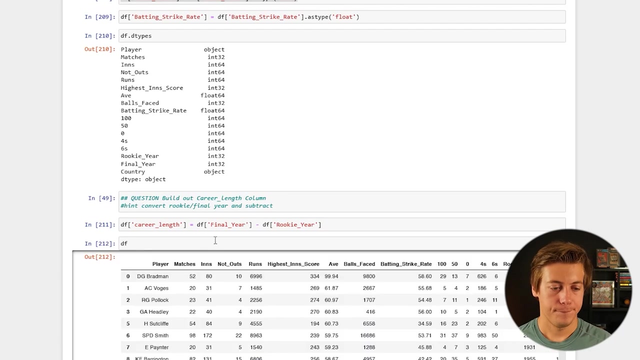 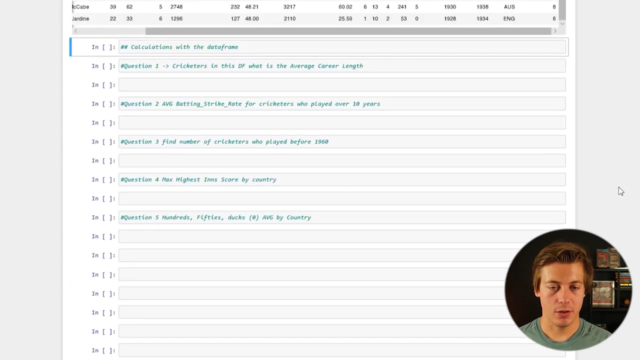 minus the rookie year And if we just run this data frame again, you can see our final year over here. career length: we have 21.7.. So we can start answering some of these questions down below. So question one: I want to see the cricketers in this data frame. 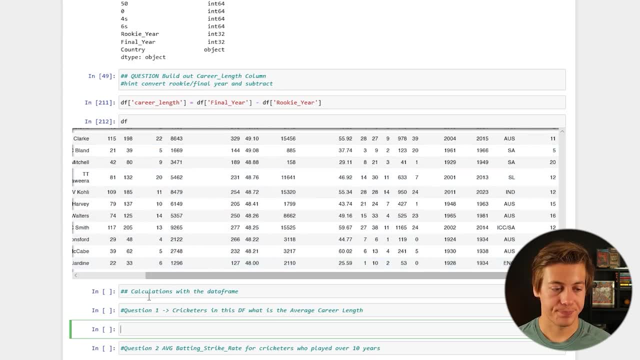 What is the average career length? And we just solve this over here. So all we have to do is df and then all you're going to do is mean: right, We run that. The average career length is 13 years. 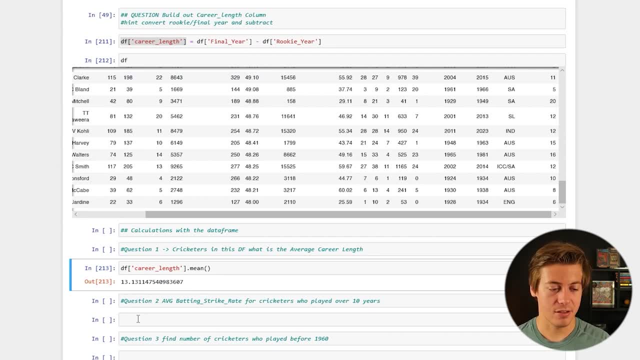 And since this is some of the best cricketers out there, it makes sense why 13 is the answer. Question two is average batting strike rate for cricketers who've played over 10 years. So you can do a few different ways. 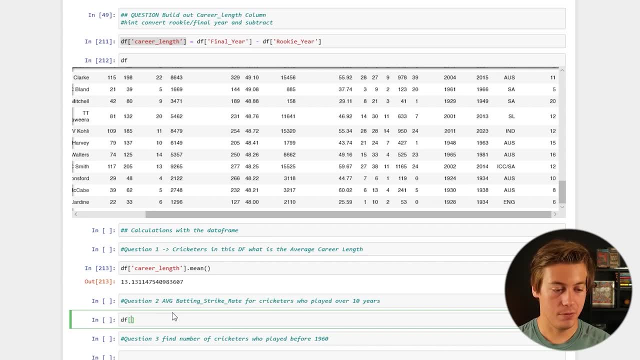 So the first one we can just do like this, pretty easy. So what we're going to do is play for 10 years, So you have career length right. Throw that in the middle has to be greater than 10, so put 10 in here. 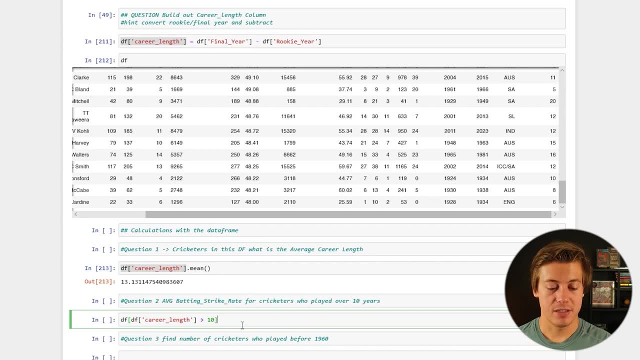 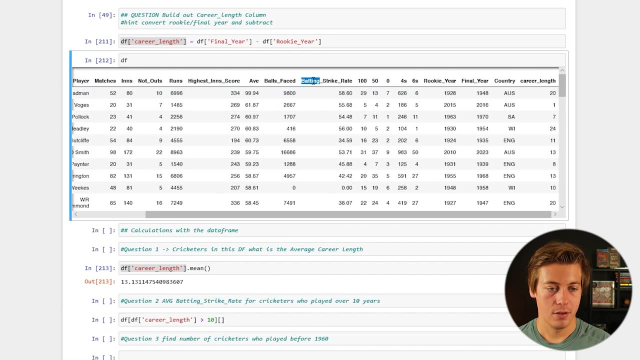 And then what we are grabbing specifically is the average batting strike rate. So we go back into these columns. We have batting strike rate, so just copy that And this will first show us- and we put single quotes around it- all the batting strike rates. 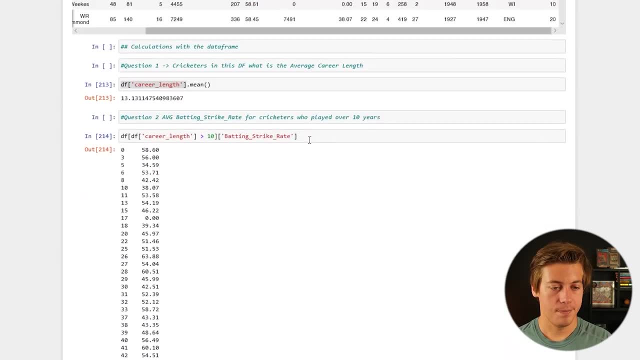 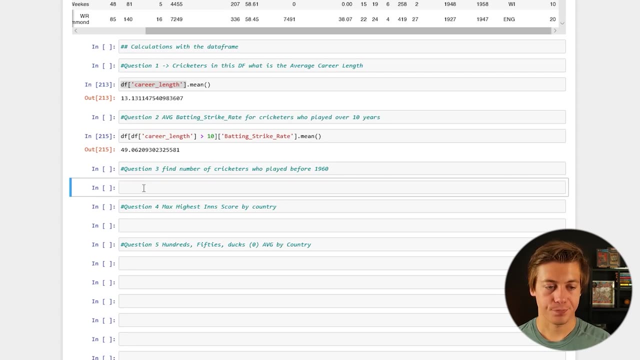 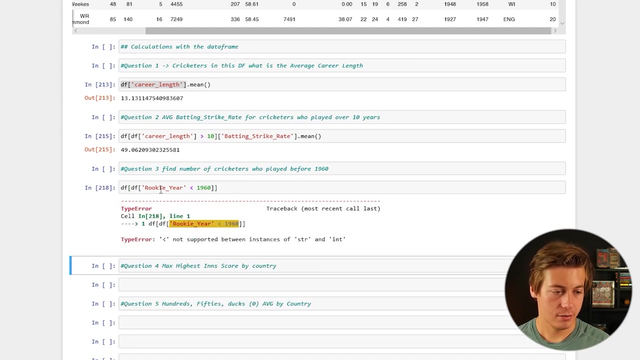 for all these people right And just put over here, mean, and it is 49.. Question three: find the number of cricketers who played before 1960, pretty easy. So df, we're going to put df, we're going to say rookie year, and we're going to say that's before 1960, and we have an error. 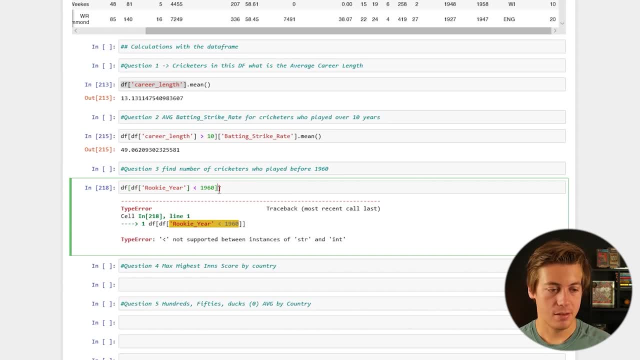 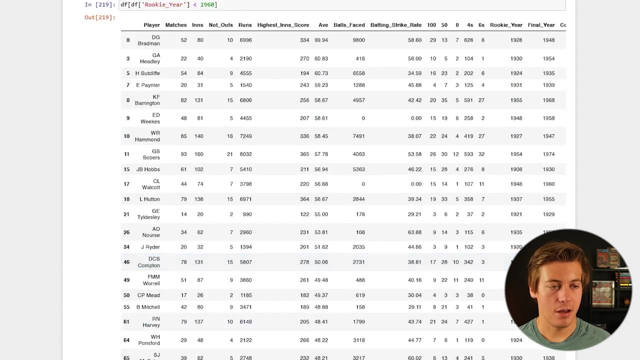 And the reason we have an error is because that is not correct And you can see all these over here, the cricketers. But now, if you wanted to find it like a specific count, you could just throw count at the end it would show you the count of each of these columns. 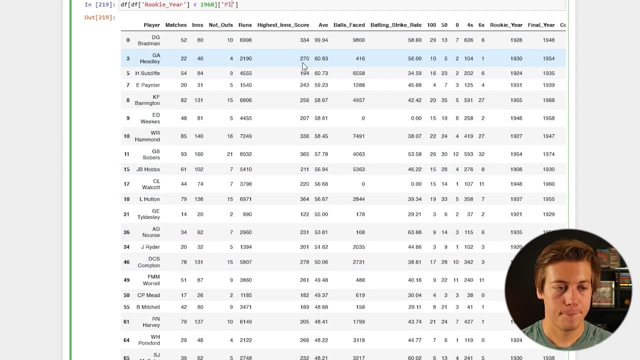 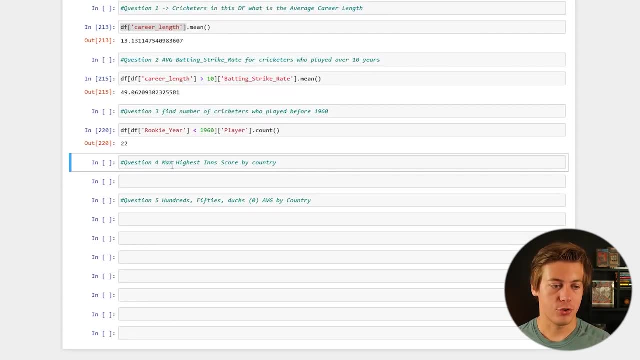 You could also just do something like this: You could do like player that counts and you can see 22 show up. So next we're going to do a group by. so it says max highest inning score by country. So, if you guys remember, we built out this country over here, so this is why we did that. 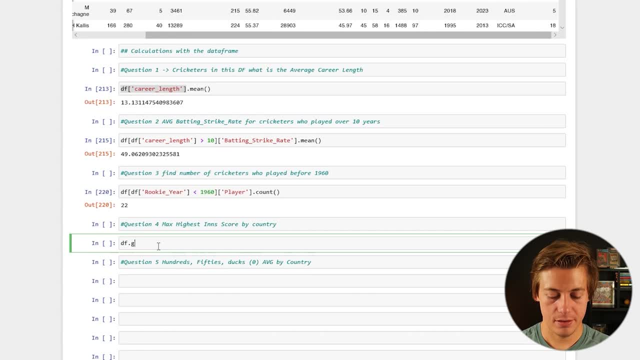 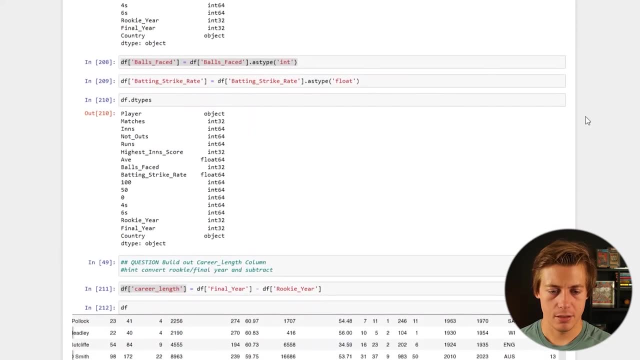 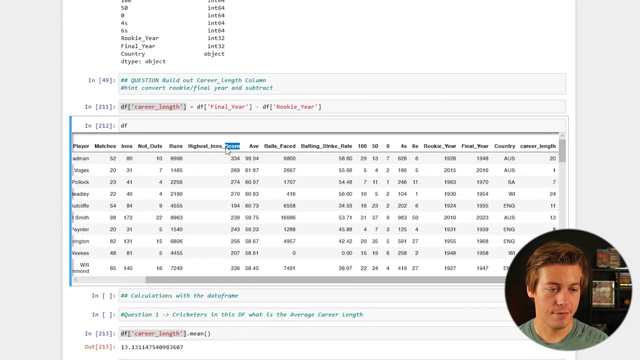 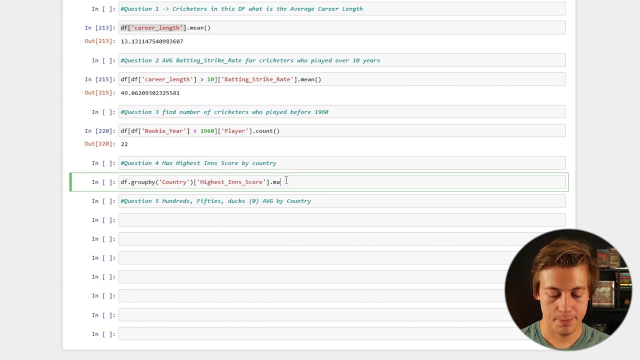 So df that group by right And then we're going to group by the country. I think it was capital C, just want to check, yeah, capital C, right, Highest inning score. so we have this over here. so just grab it, that's, and then just put max, so max, and you can see specifically how these rank. 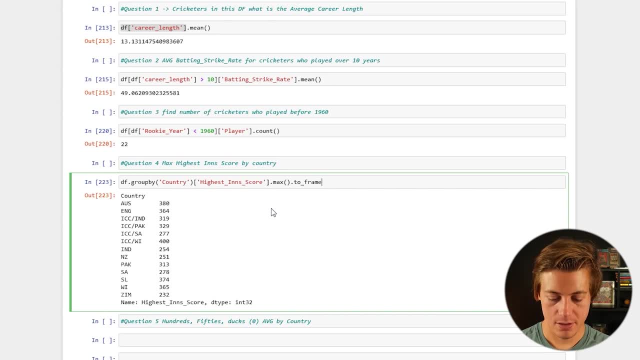 But if you wanted to sort them, I'm just going to say two frame first and we're going to say this is High in country, something like that. I don't know doesn't really matter, And then reset index that and then sort values and then just throw this in here, right? 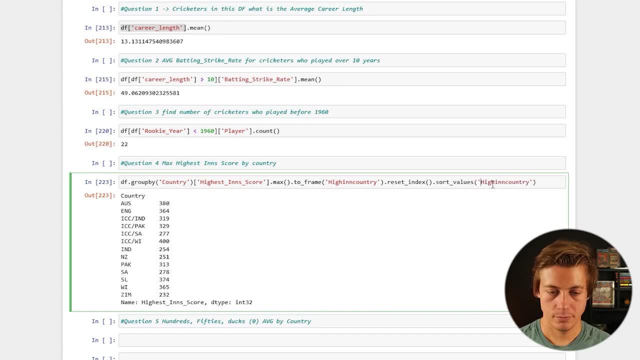 And then you can see how that works. But if you want to change the direction, you can say ascending. you can also change it to higher. What we're going to do is just take this over here and we're going to go through it every time. 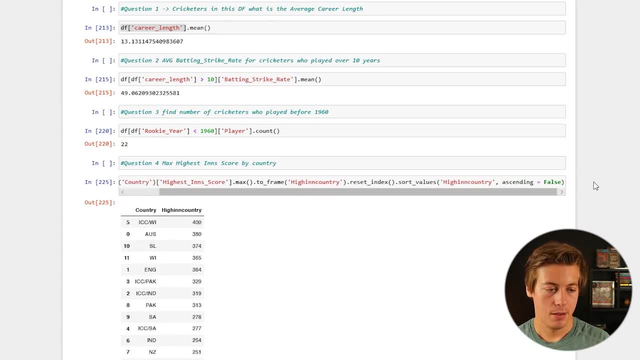 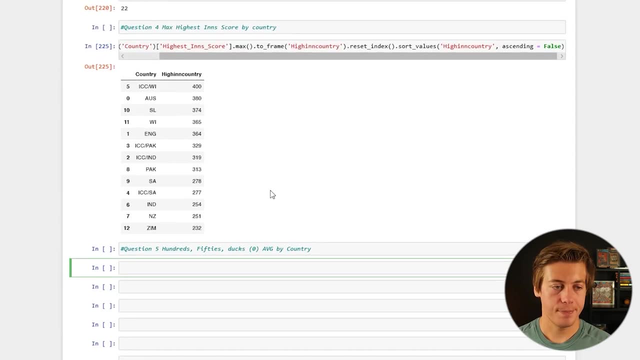 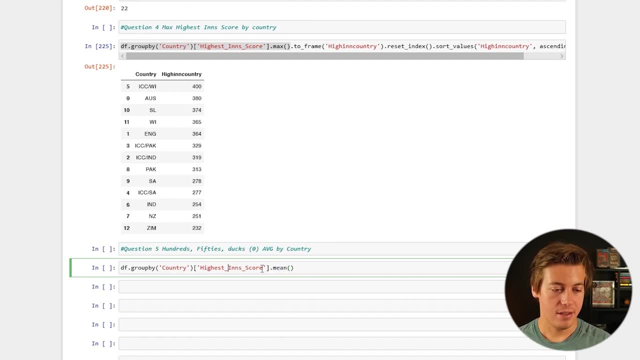 first we're going to change this into mean and then this needs to be changed. so, since we're grabbing multiple, a series is now i'm going to do it like that, and first one's going to be 100, next we're going to have 50, next we're going to have zero and then dot mean, like that. 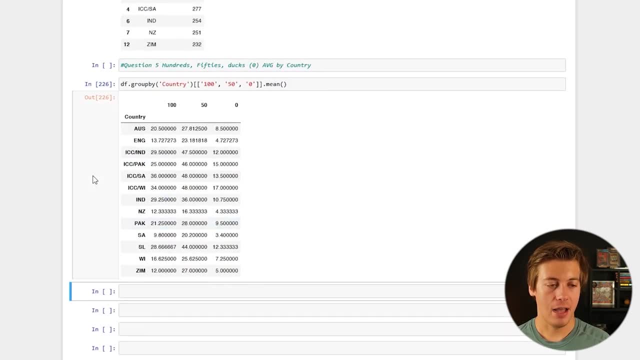 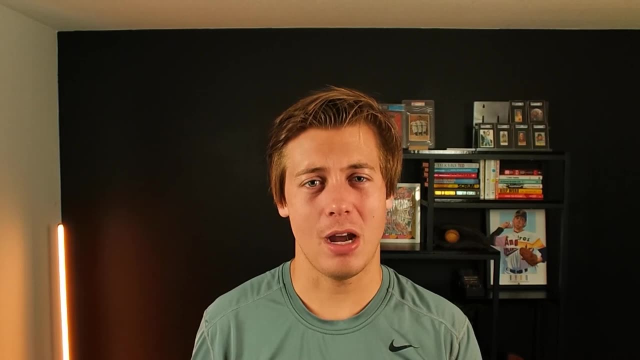 and then you can see the average for each of these different countries. hope you found this video helpful and also you learned a few new things, if you did make sure to subscribe to the channel. i really recommend, though, that you check out this video over here, where we solve. 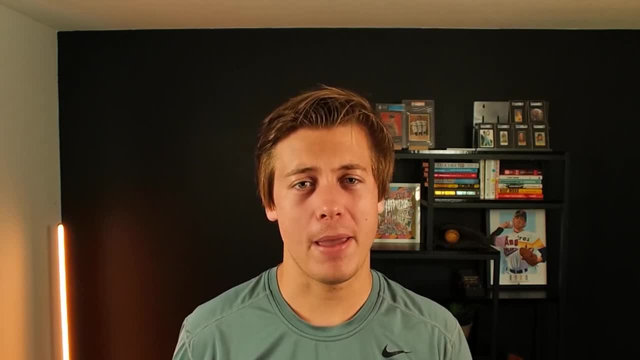 some python interview questions you because it mainly uses pandas.